Greetings to everyone. Welcome back once again to my educational channel on biology. I'm Teacher Janet and today let's discuss a whole chapter from Form 5 KSSM Biology Syllabus. The title is Adaptation of Plants in Different Habitats and this is Chapter 7 in the Form 5. 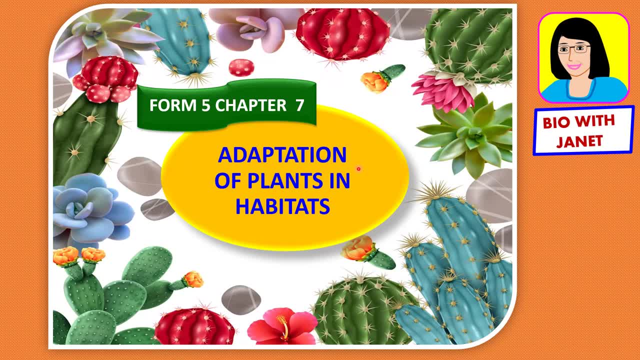 Biology Syllabus. So it's interesting to discuss what types of special or unique features that plants have in relation to the habitats in which they are living, so that they can adjust to the conditions in the different habitats in order to survive and also to grow healthily in these. 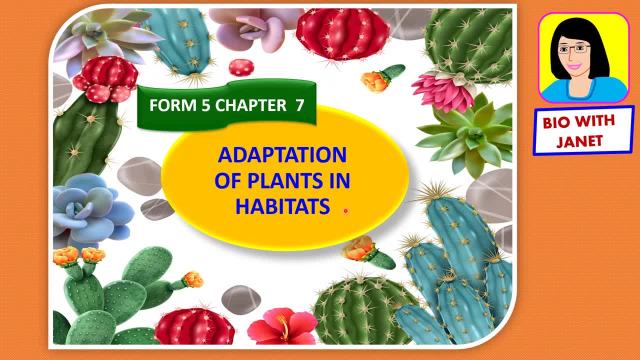 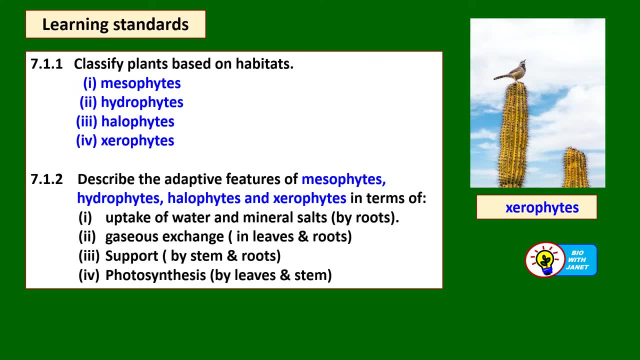 habitats. Let's find out more about the different habitats and what are the classification of plants in different habitats. So let's get started. The learning outcomes for today's lesson are as follows. Firstly, we should be able to classify plants based on their habitats. 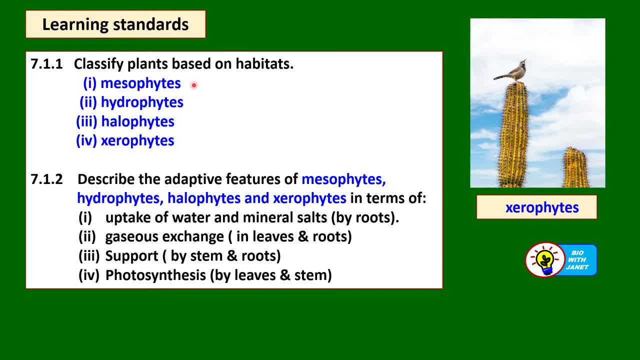 So there are four different types of plants that grow in different habitats: Number one, mesophytes, Number two, hydrophytes, Number three, halophytes And number four, xerophytes. Next, we should be able to describe the adaptive features or adaptations. 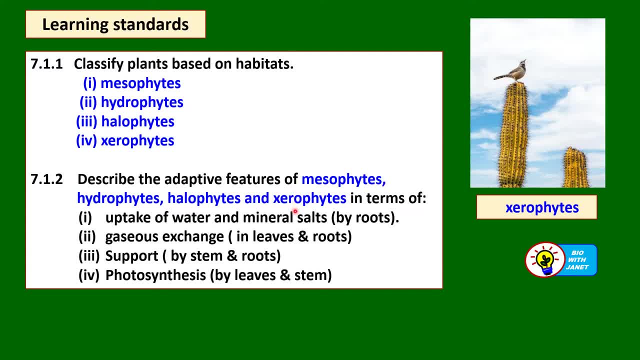 of mesophytes, hydrophytes, halophytes and xerophytes in terms of number one uptake of water and mineral salts. So this is carried out by the roots. gaseous exchange in leaves and roots. 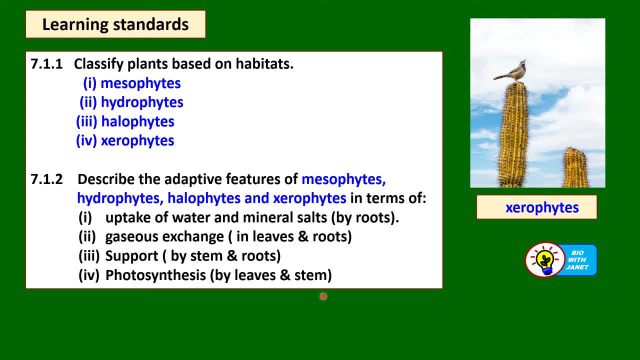 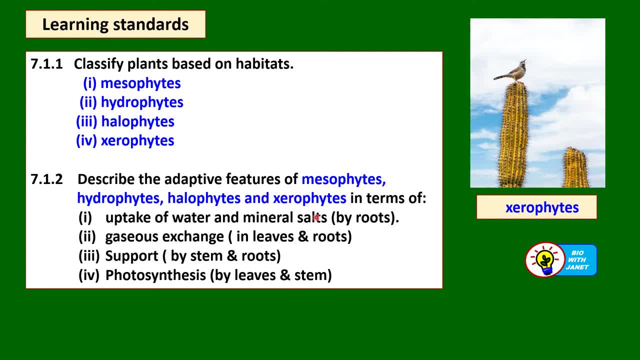 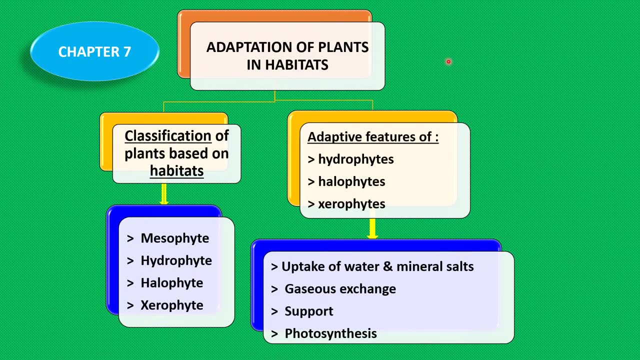 discuss these adaptations of the different plants in their different habitats. So it's very interesting to find out how they are adapted to live in their different habitats. Here's an overview of what we are going to discuss: Adaptation of plants in different habitats. First, the classification of plants based on their habitats. So we have four different. 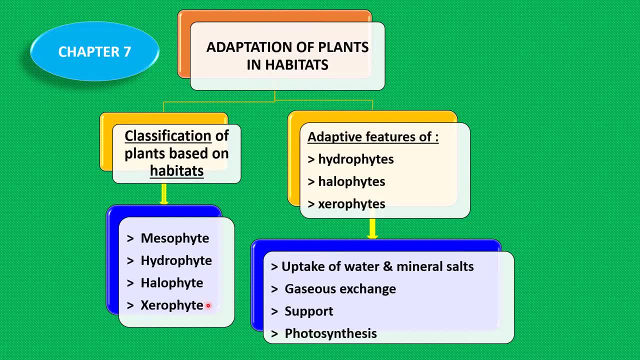 types of plants: mesophytes, hydrophytes, halophytes and xerophytes. After that, we're going to discuss the adaptive features of hydrophytes, halophytes and xerophytes. Mesophytes: 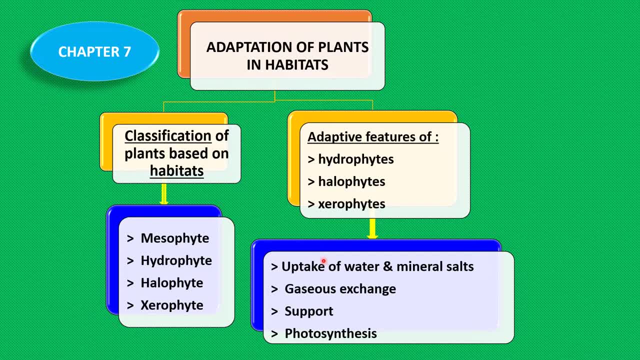 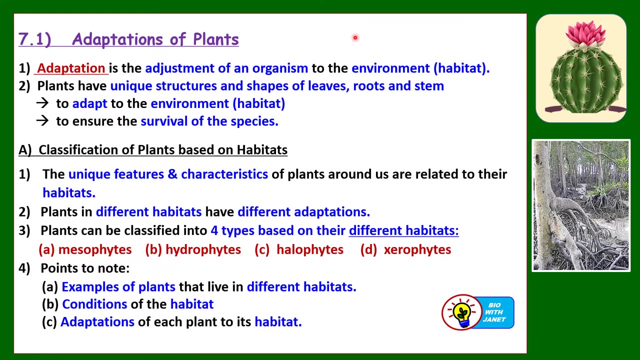 is not included, right, And so we are going to relate the features to the processes that they have to carry out, like uptake of water and mineral salts, gaseous exchange, support and photosynthesis. So the title of this topic is the adaptations of plants in different habitats. Now what's the 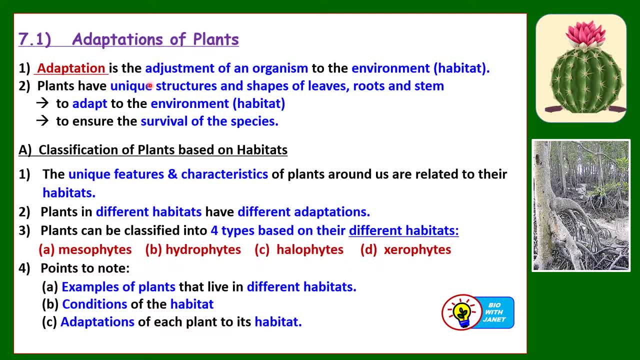 meaning of the word adaptation. Adaptation means that the plant is adapted to live in different habitats. That means the adjustment of an organism to the environment or the habitat in which it lives. So plants have unique structures and shapes of leaves, roots and stem to adapt. 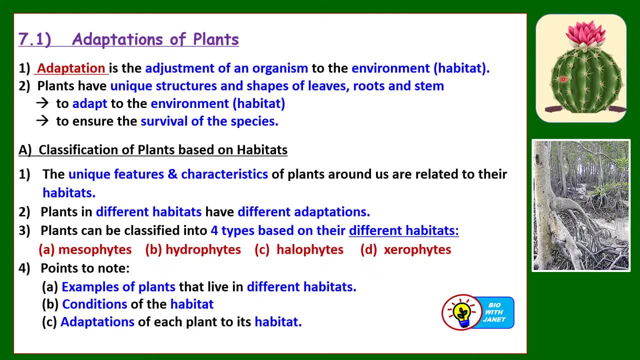 to the environment in which they live or the habitat in which they are living in, to ensure the survival of the species. For example, when we look at this type of cactus- right, you know it's a cactus, it has a rounded shape and there are no leaves on it. okay, just a. 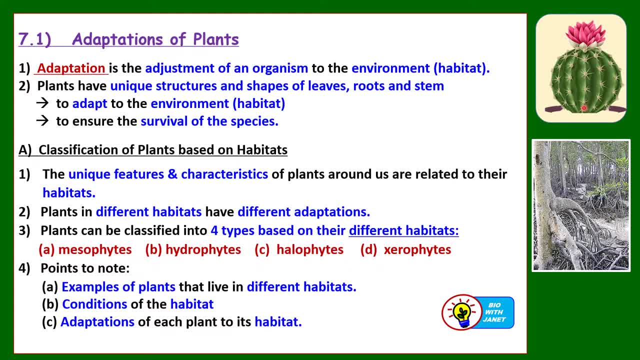 stem that is very round, right? So? and then the leaves are modified to form thorns. So why is it like this? So that's the reason: because it lives in the desert, right To conserve water and also to store water in its stem. That's why the stem is so big and round. So another one is the mangrove. 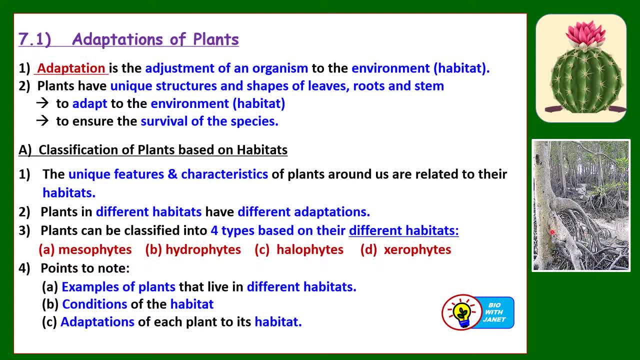 swamp. We can see trees like these in the mangrove swamps, with roots that stick up from the ground, spread out in this way, right. So this is more for support in the environment in which they live, which is the muddy conditions near the seashore. So let's find out more and relate and try to find. 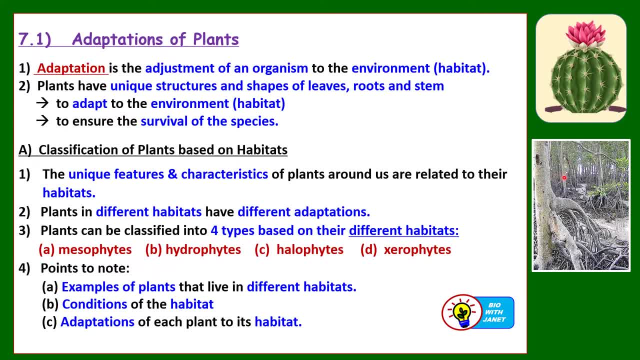 out the reasons why different plants have different unique characteristics, structures and shapes of leaves and roots and stem, And how is it related to the environment in which they live, to the physical conditions that they face? Right, that's very interesting to discuss. So a classification of plants based on habitats. So 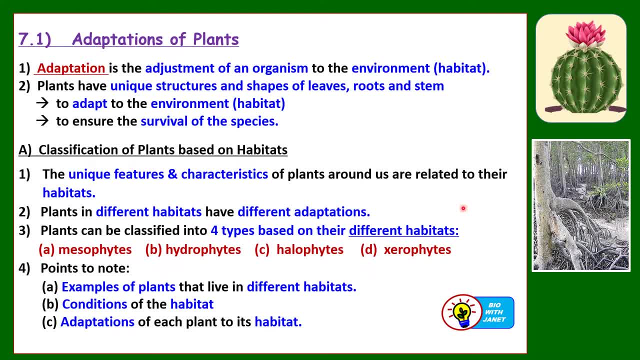 unique features and characteristics of plants that are observed around us are related to the habitats, and plants in different habitats will have different adaptations. So there are four types of plants based on the four different habitats that we're going to discuss. Okay, the plants can be. 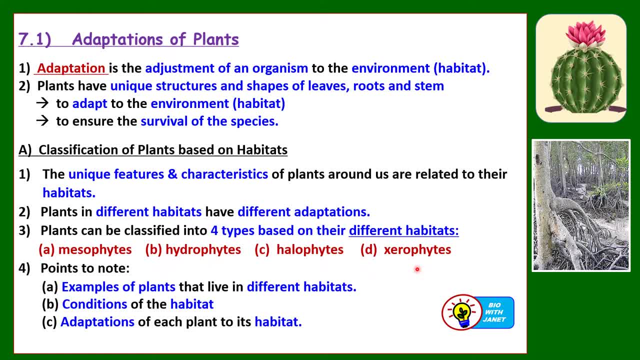 classified as mesophytes, hydrophytes, halophytes and xerophytes. So the points that we're going to note are examples of plants living in the different habitats, and then the conditions of the habitats and how each plant is adapted to the conditions in the habitat. 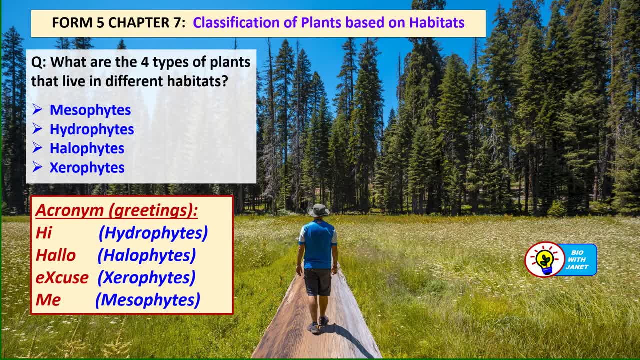 So what are the four types of plants that live in different habitats? Right, we have discussed that just now. We have stated the names, So mesophytes, hydrophytes, halophytes, xerophytes. Now I'll give. 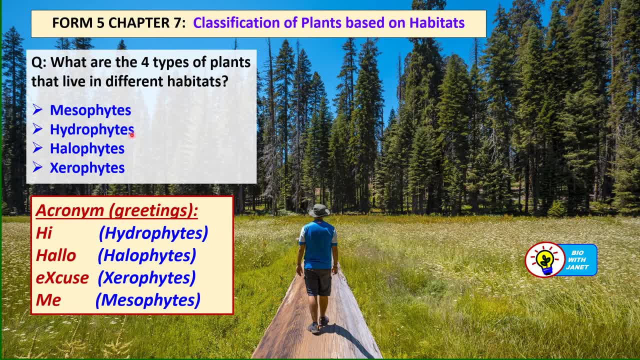 you an acronym here which is very easy to use For hydrophytes. we have to the word. we have the word hi For halophytes. hello to remember it. xerophytes xq. X for zero, x for zero. 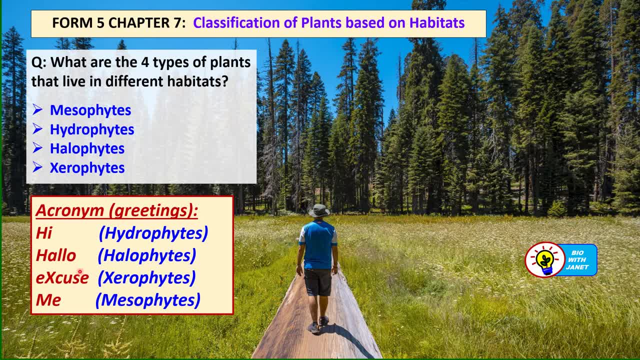 And me for mesophytes, right? So hi, hello and excuse me, These four greetings and words that we say to another person, this form the acronym for the four types, four different types of plants that live in different habitats. righteous plants. 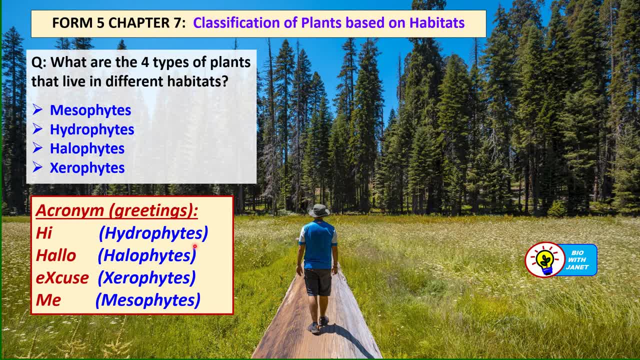 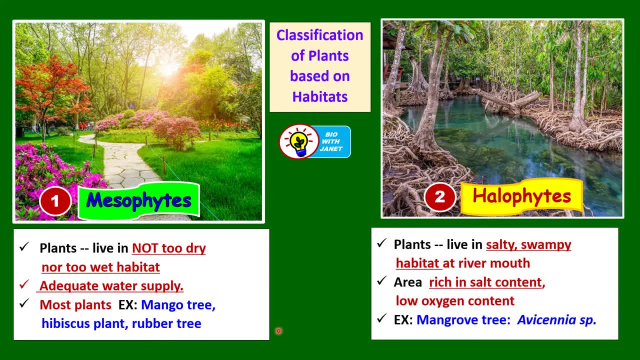 different habitats. Hi, hello, excuse me. Okay, so you can use this acronym to remember these four types of plants. Let's discuss the classification of plants based on their different habitats. So there are four types of plants. Firstly, the mesophytes. Mesophytes are plants that live in. 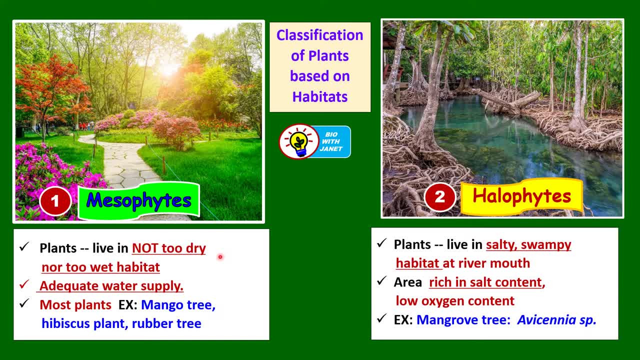 moderate conditions, that is, conditions that are not too dry, not too wet, and their habitats have adequate or sufficient water supply. These include plants such as fruit trees like the mango tree, rambutan tree, durian tree, then flowering plants such as hibiscus plant and rubber trees. 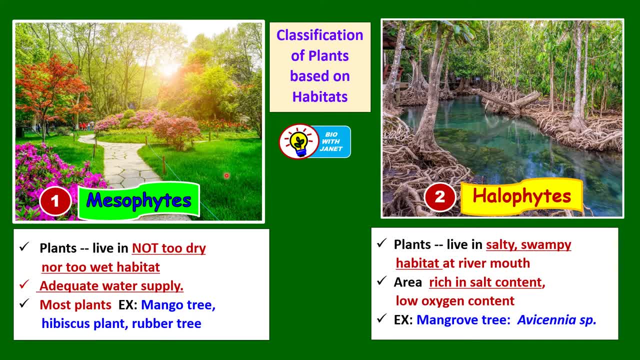 and other types of trees, including the grasses, as seen here. So we see that the mesophytes are not too dry, not too wet, and their habitats have adequate or sufficient water supply. So we see these plants in the school field, in the parks. 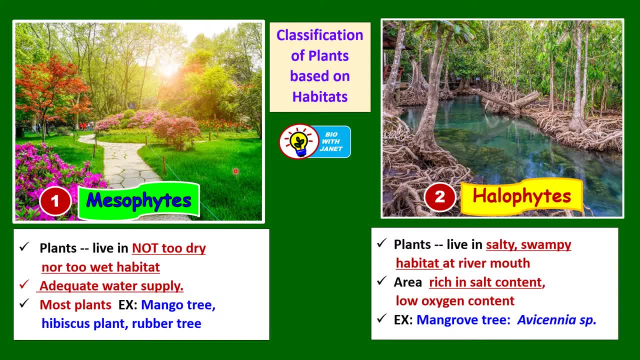 and in the residential areas, in the gardens around us. Now, the second type of plant are called the is called the halophytes. Halophytes are plants that live in the salty or swampy habitat at the river mouth near the sea, and this area is rich in salt content. Also, the mud has low oxygen. 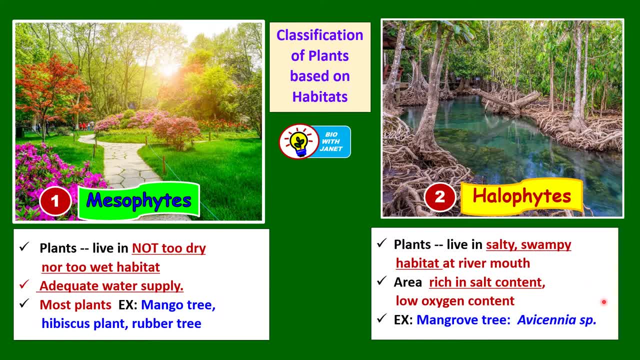 content here. So halophytes are trees or plants that are well adapted to live in the swampy conditions and they are very special adaptations. Examples are mangrove trees and other trees. So an example of the mangrove tree that we have to know is every senior species. 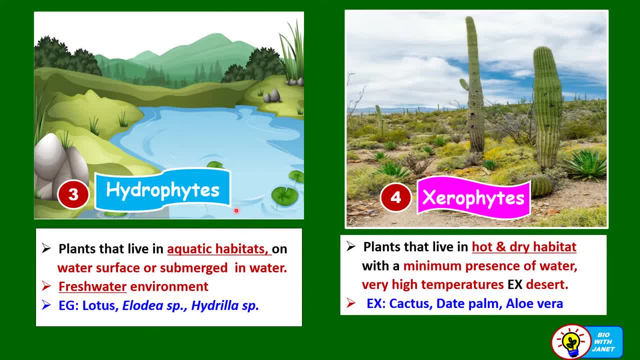 The third type of plant are the hydrophytes. Hydrophytes live in aquatic habitats. They live on the water surface or submerged in the water. For example, we can see some of these leaves here. These are water lily plants, all right, and they either float the plants either float on. 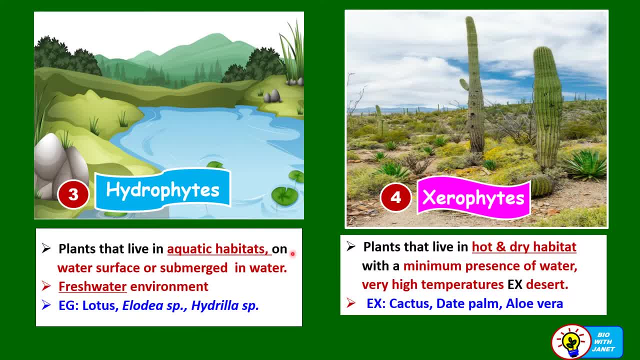 the water surface or they are right inside the water, submerged in the water, And then this is a freshwater environment because of the water here, which has a low concentration of mineral salts compared to salt water, So it's called freshwater. The water in ponds and lakes are. 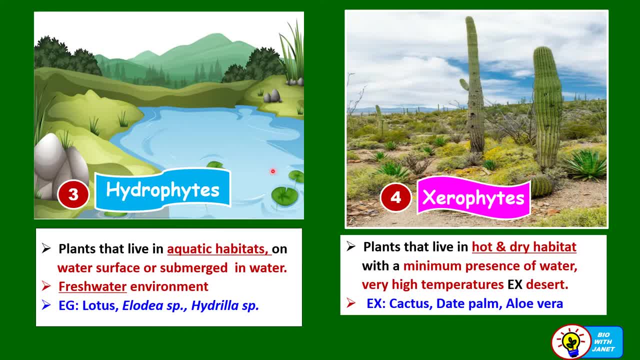 freshwater. Examples of plants living here are the lotus, this is the lily, and then elodea species and hydrilla species are submerged in the water. Now the fourth type of habitat is the dry hot conditions. It's a habitat with hot and dry conditions, and xerophytes live in the 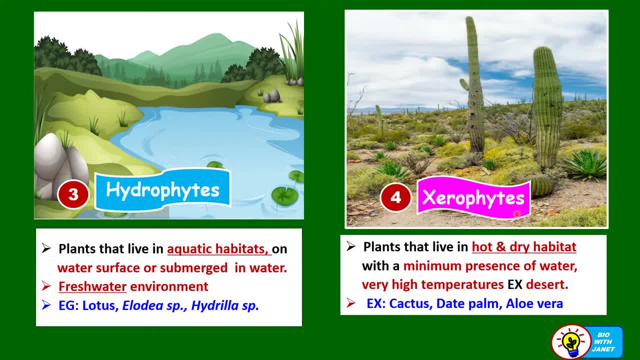 hot and dry habitat which have a minimum presence of water. That means they have a lack of water, very high temperatures, such as in the desert. So we know that cactus, or cacti, live in the desert, together with other plants like the date palm and aloe vera plant. 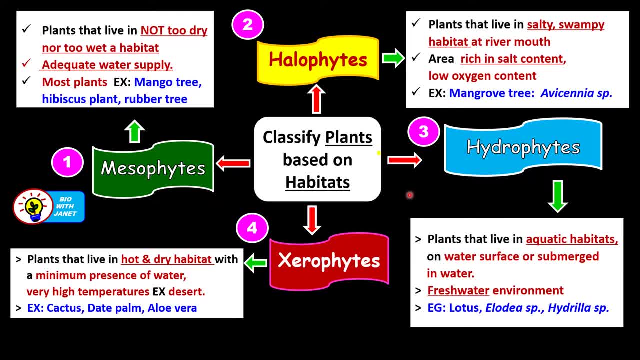 So here's an overview of what we have discussed in the previous slides: Classified plants based on the habitats. So there are four types of plants: The mesophytes that live in more dry, humid conditions. The word meso means middle right. We have already discussed the examples. 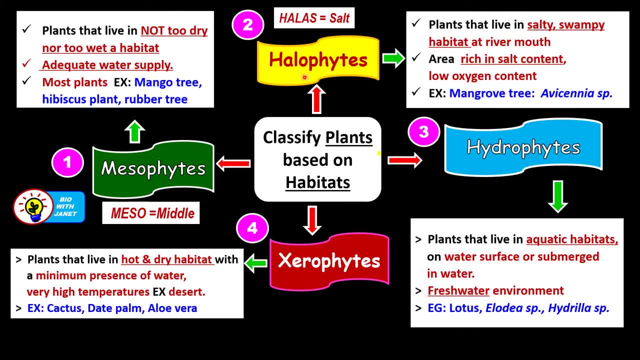 And then halophytes, from the word halas, meaning salt. Halophytes from the word halos, from the words halas, meaning salt, So these plants live in the salty, swampy conditions, And examples are the mangrove trees. Then we have the hydrophytes: Hydro means water, So these 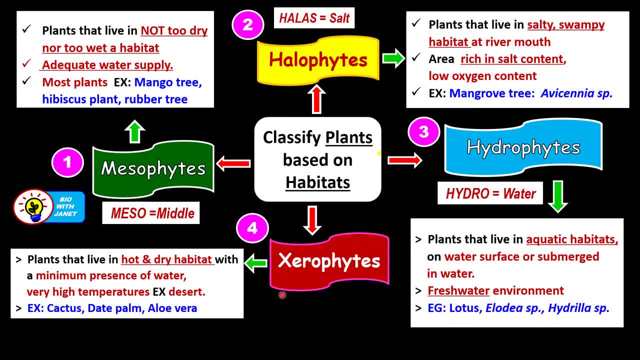 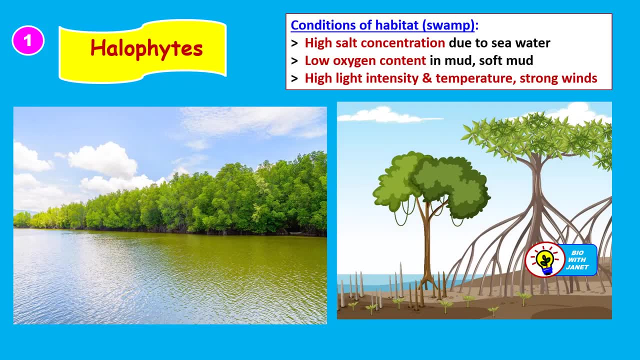 plants live in the freshwater environment. Examples are the lotus. And then we have the plants living in the hot, dry conditions. The word zero means dry, So you can copy these notes into your notebook. Next, let's look at three types of plants. We will not talk about the mesophytes that live in moderate conditions. So 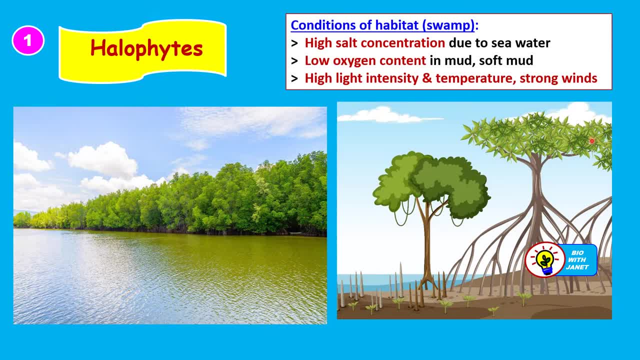 let's look at the halophytes Now. halophytes are plants that live in the swampy region, near to the sea, At the river mouth, near the sea. So the conditions of the habitat is that there's high salt concentration right in the water near the sea And then a low oxygen content in the mud. 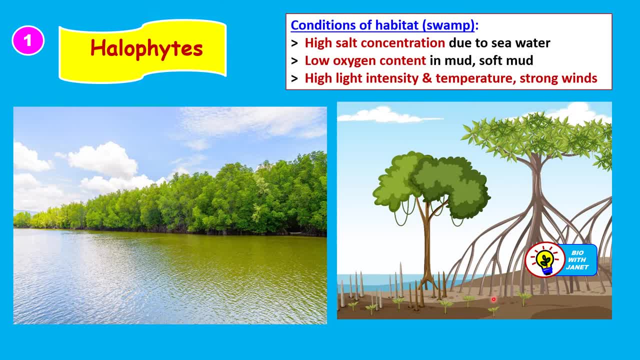 because the mud, the water in the mud, has displaced the oxygen out of the mud. Okay, And these kind of places have high light intensity because they're exposed to the sun And high temperatures. They're very hot And also strong winds from the sea blowing to the sea or from the sea. 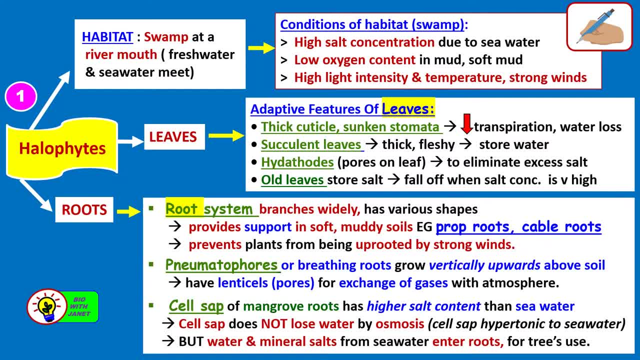 This schematic diagram shows us the adaptations of the halophytes for its habitat, which is the swampy area at the river mouth where fresh water and seawater meet. Conditions of the habitat or swamp: There's high salt concentration due to the sea water And there's a low oxygen content in the mud. Furthermore, the mud is very soft. 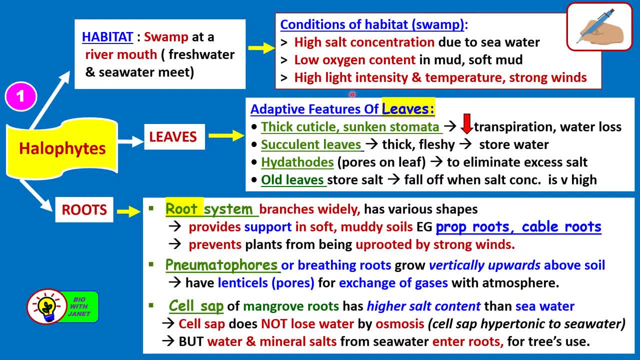 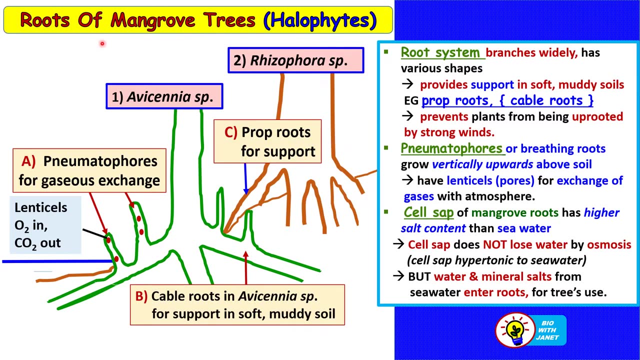 And then there's high light intensity and high temperatures, with strong winds. So we are going to discuss the adaptations of the leaves and the roots. So you can copy this schematic diagram into your notebook if you want to. Now, firstly, we're going to talk about the roots, So the roots of mangrove trees are very special. 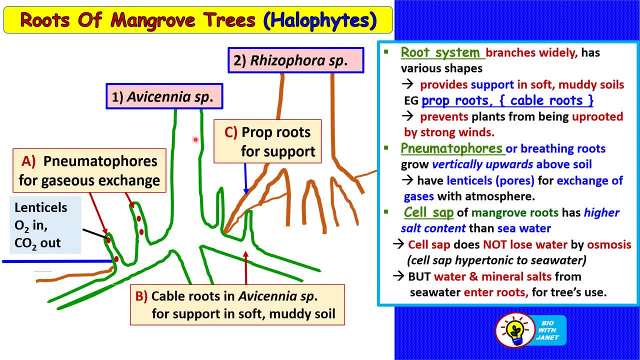 Okay, they're halophytes, And here we see two types of plants or trees which are called the abyssinia species and the rhizophora species. There are two types of mangrove trees. Now, in another chapter coming up, we will be studying the specific adaptations of these. 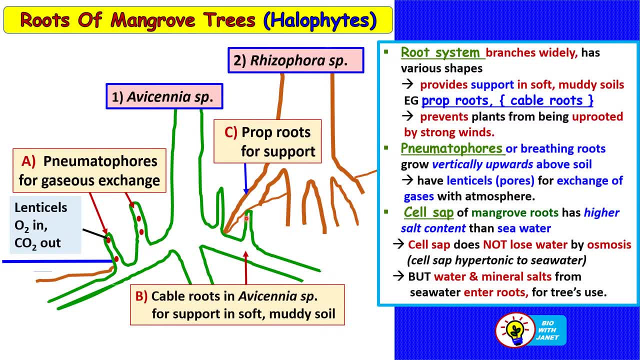 mangrove trees, Right. So here we just studied generally And let's look at first of all the root system. So root system branches widely and has various shapes, So the first adaptation is to provide support in the soft, muddy soil. Right, For example, there's the prop root and the cable roots. Okay, let's discuss this first. 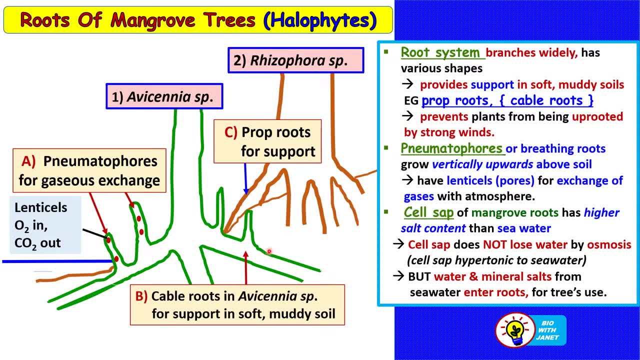 adaptation, which is the branching out of the root system to provide support in the soft, muddy soil here. So let's look at rhizophora species. It has roots that project out above the surface of the ground like a tripod, stand spread out onto the ground like this. 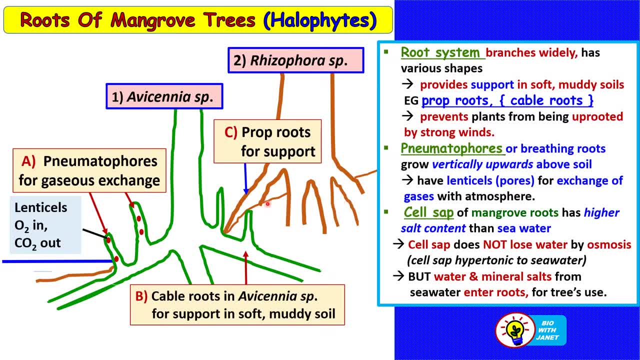 So this provides a broad surface area underneath Right Now, and this will allow the roots to give more support to the soil, just like if you put your hand on the table but raise it up a bit and spread out your fingers and then push it down on the table. It's very stable, Right. 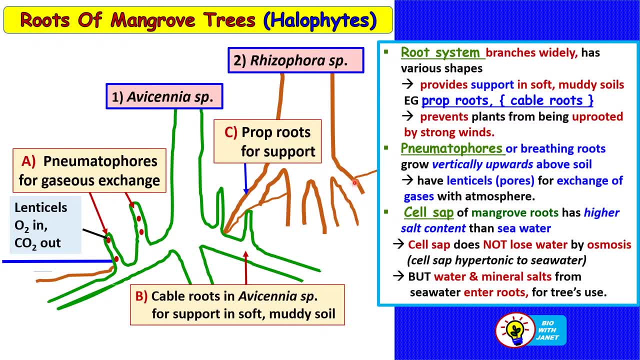 So this is the type of support now that is provided by the prop roots. It's called the prop roots Right. This this looks like fingers. You spread your fingers- table, for example. like this right. it gives a lot of support. so this is the. these are the. 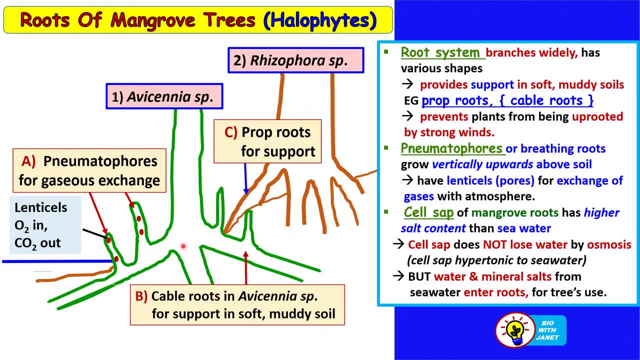 prop roots, and then we have the cable roots. now, cable roots are found in every senior species and they are horizontal and under the ground, under the soil, under the mud, unlike the prop roots that are above the mud. okay, so the cable roots are under the ground, near the surface of 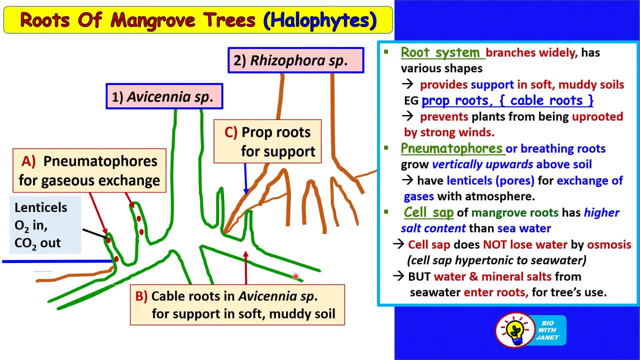 the ground, but underground, near the surface, and it spreads up horizontally in different directions from the tree trunk. so, again, this gives a broad surface area of the roots and this helps the plant to be supported- well supported- in the soft, muddy soil right. then, also, by providing the support, it prevents the plants from being uprooted by the strong winds. 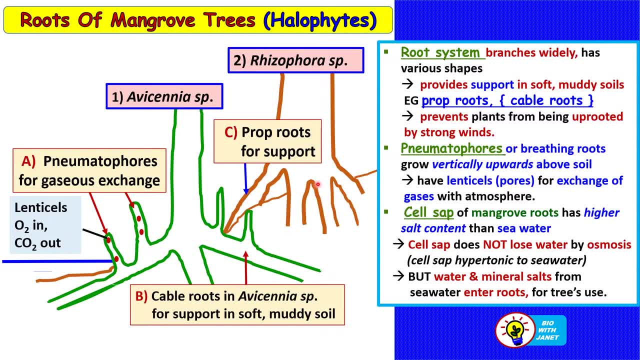 that blow in from the sea as an example. so that is the first type of root, the roots that give support. now there's another type of roots, which are vertical. they stand out vertically above the ground, so these are called pneumatophores. pneumatophores, or breeding roots, grow vertically upwards, above the 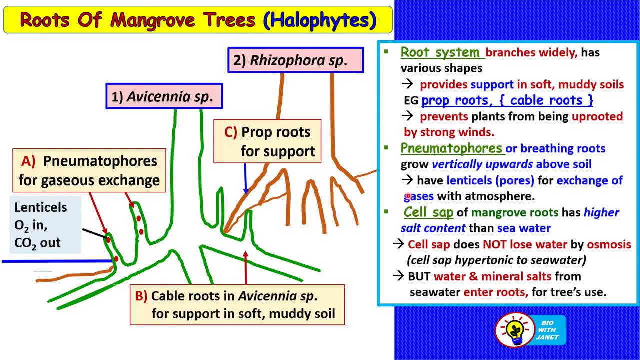 soil and they have lenticels or pores for the exchange of gases with the atmosphere. so let's have a look at the pneumatophores. pneumatophores- here now they stand up vertically and then on the vertical roots. here the pneumatophores. 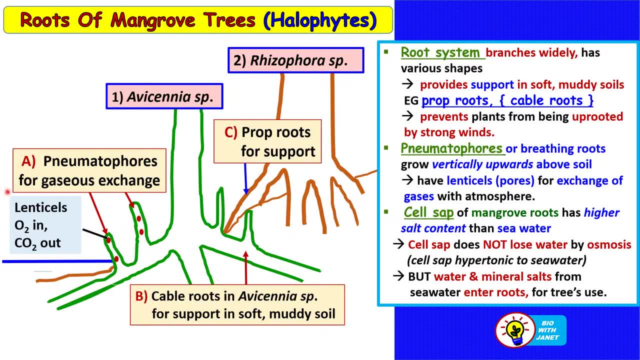 there are pores or holes to allow oxygen to diffuse into the roots. so once oxygen gets into the pneumatophores it can also be carried to other parts of the roots which are below the ground in the soft mud. so in the soft mud there's a lack of 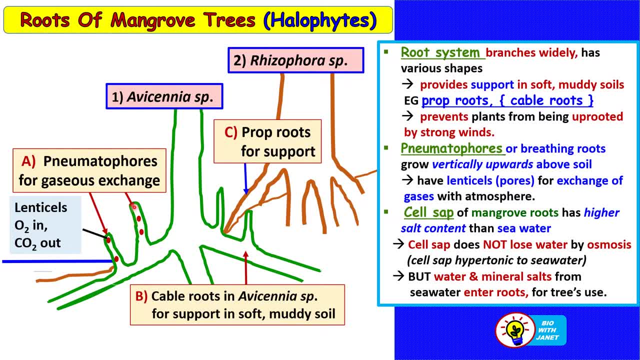 that's why there needs to be pneumatophores. okay, the word pneuma means air, so it is to obtain air from the, the environment above the mud, and then you can channel down, channel it down to the roots below, okay, so pneumatophores are actually vertical breathing roots that are important for gaseous. 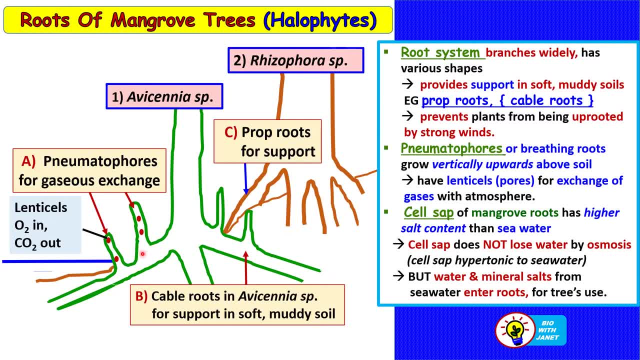 exchange between the roots and the environment and they grow vertically up above the soil, above the mud. they have lenticels for to allow oxygen to diffuse into the roots and carbon dioxide to diffuse out. so that is the adaptation of the roots to obtain enough oxygen from the air, since they 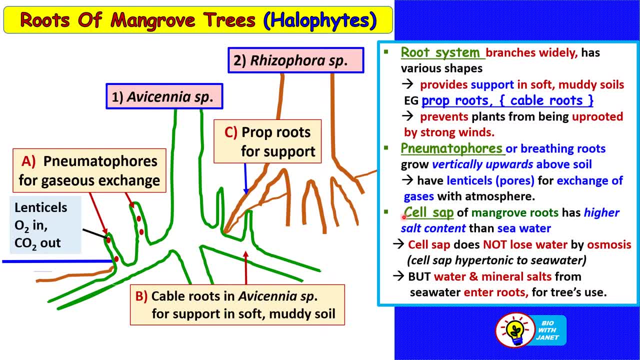 live in the muddy soil now. next, we have the cell sap. cell sap in the mangrove roots here, which are below, below the sea level and sometimes the sea, you know. the tide will come in and it will cover most of the roots, right then what happens is that the salt water tends to be have a high 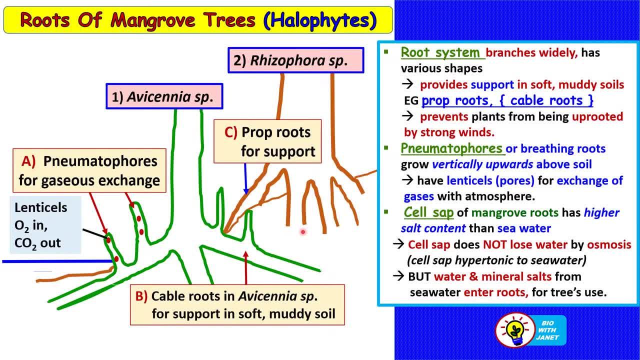 concentration of salt. so it would tend to draw water out from a normal tree. but not so for the mangrove roots because the cells- cell sap of the mangrove roots are the main source of the mangrove roots- has higher salt content than sea water and the cell sap does not lose water to the sea, to the. 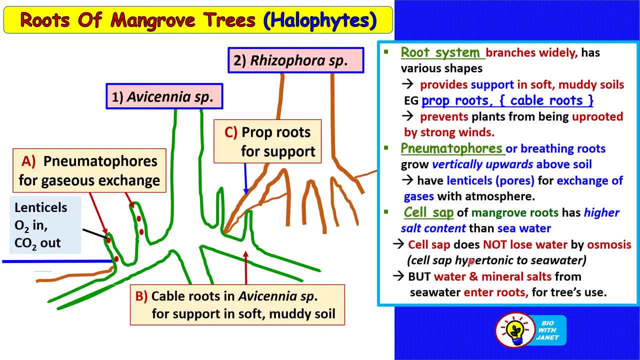 sea water by osmosis, because the cell sap has a high concentration of salt, so it is hypertonic to the sea water. so water will diffuse from a hypotonic solution to a hypertonic solution. thus water will diffuse from the sea water, which is more dilute. okay, then the cell sap, so it's 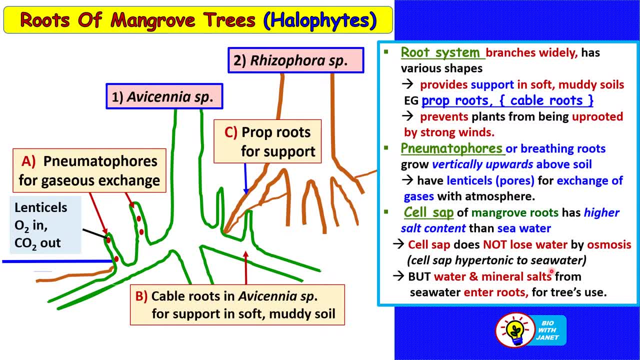 more dilute. okay, then the cell sap, so it's more dilute. okay, then the cell sap, so it's more dilute. okay, then the cell sap, which is hypertonic to the sea water. so water, mineral salts from sea water enter the roots and can be used for the trees use, okay. so the only problem is this tree will have a lot of. 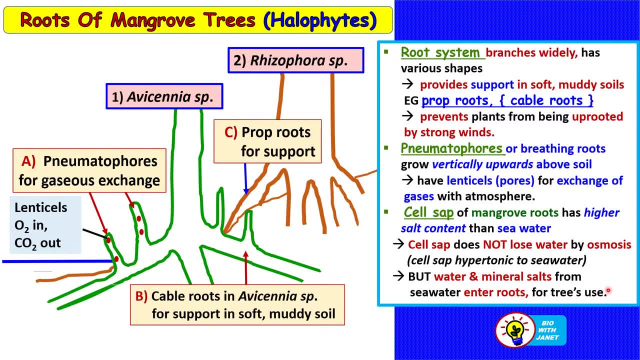 salt in it and let's find out how the salt is excreted from the tree. so, basically, there are three features that we need to know about the mangrove roots, as the mangrove roots are the ichromuscles that are cultivated yearly, so a mangrove has two different cell groups. 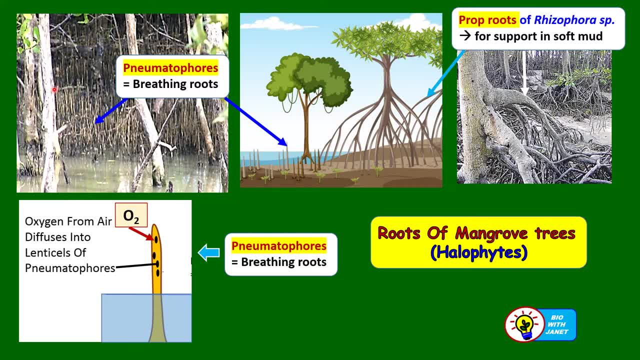 first one that's called Phala. any last root, though, it's called Phala, as always a South African one known as Phala, the most important whole. so that's one feature of this mangrove, such as shingles, one known as Phala أن orphanes. 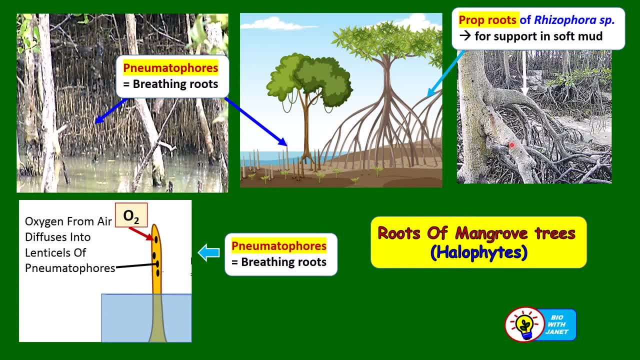 two other type of marine widespread. you want to know more about phala. let me show you when I went on an expedition or a trip to a mangrove swamp in Perak state. So these are the mangrove trees with the prop roots, rhizophora trees. 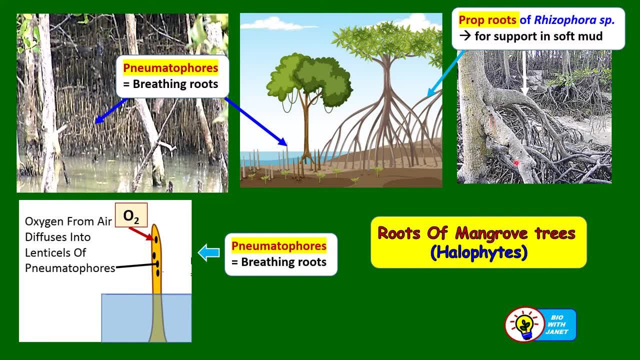 Prop roots stick out from the tree trunk above the mud, but it provides a broad base below for the tree to obtain support so that it does not topple over. And here you see the pneumatophores, as is shown here, where there are holes or pores, called lenticels, for oxygen to diffuse into the roots. 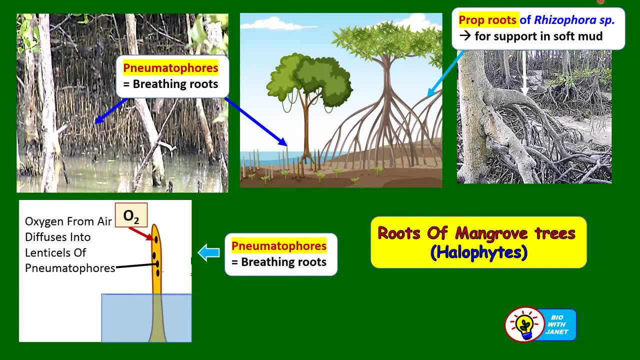 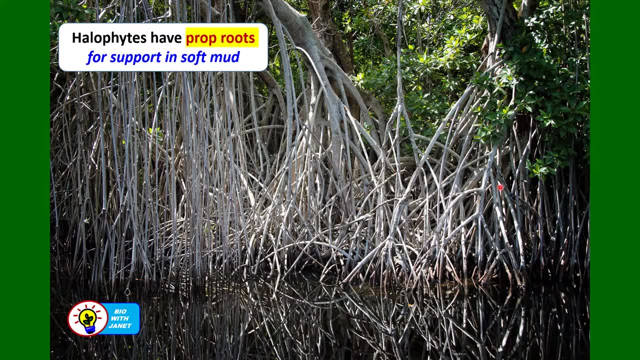 So the nodes are the same. it's just now. So what types of roots are these? Now, this type of root are the prop roots also found, also photographed, from the tree in the mangrove. So this type of roots are for support in the muddy soil. 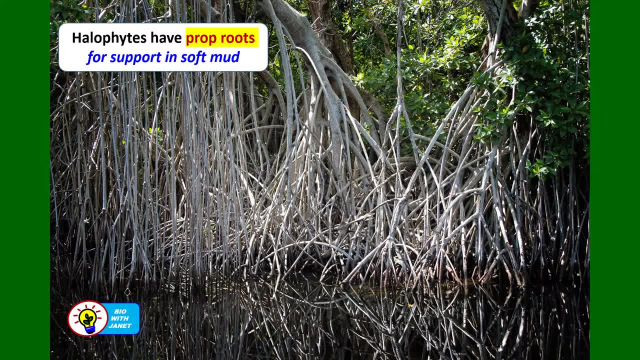 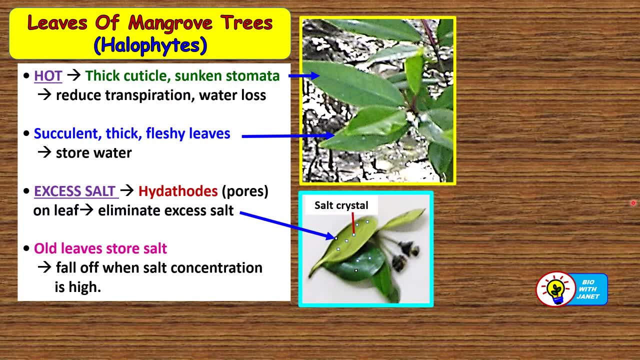 and also prevents the tree from being uprooted by strong winds. Now let's discuss the leaves of the mangrove trees. So the leaves have to reduce transpiration and they do so by having a thick cuticle and sunken stomata, which we will discuss afterwards. 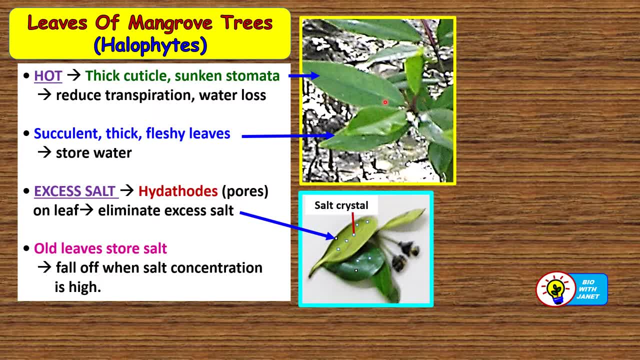 So the cuticle on top of the leaf, the waxy cuticle, is dry, Thick And when we look at the leaves they tend to shine in the sunlight because of the waxy cuticle. So this waxy cuticle will prevent evaporation of water by transpiration. 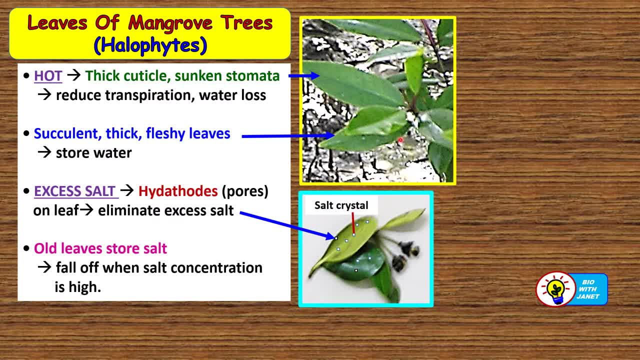 from the leaf cells to the atmosphere, So it reduces water loss. Secondly, the leaves tend to be thick and fleshy, Or we say succulent. Succulent means that it's thick and fleshy because it stores water inside. That's why it's thick and fleshy. 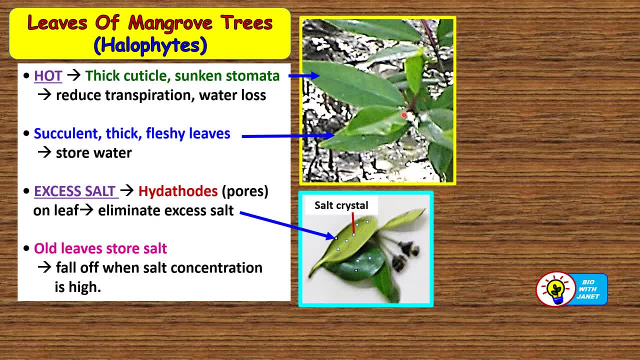 Thirdly, on the surfaces, on the top part of the leaf and also the bottom surface of the leaf, there are hydratodes or pores or holes to eliminate the excess salt inside the plant. So sometimes you can see some whitish substance on the tree leaf. 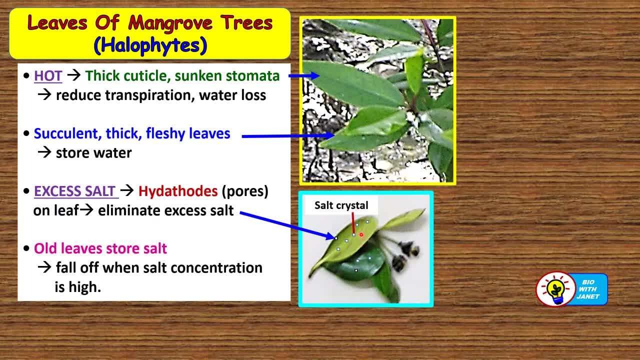 either on the underside or at the top, And this whitish substance are actually the salt crystals, Because salt is eliminated or excreted through the hydratodes or pores on the leaf which are found on the leaf surface. Another way to get rid of salt is that the old leaves 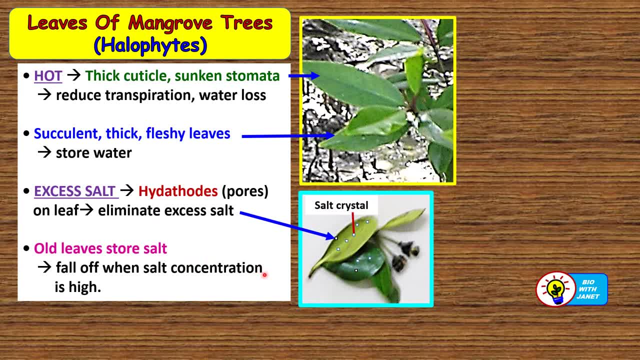 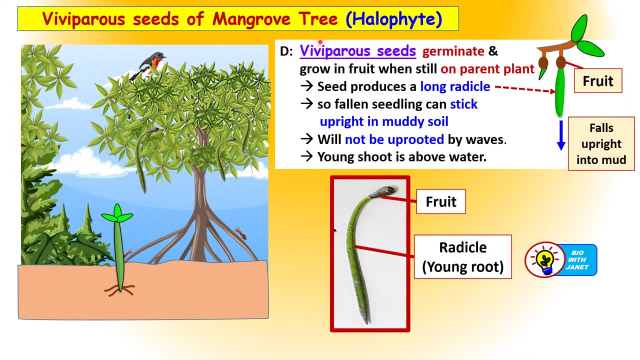 mature leaves will store a lot of the salt And then they will fall off when the salt concentration is high. Next, let's discuss the seeds of the mangrove tree. So mangrove trees have a lot of seeds. They have viviparous seeds, which are very special. 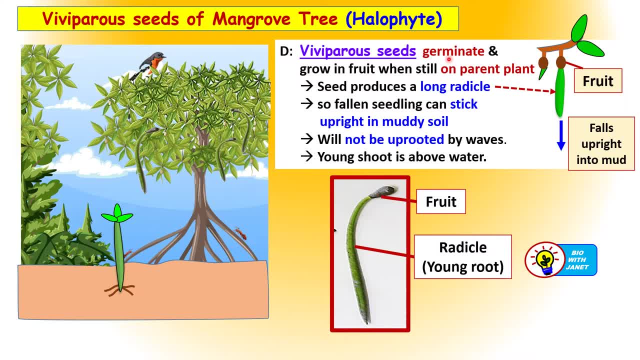 This means that they germinate and grow the roots, the root system, while they are still inside the fruit on the tree. That means they germinate while they are still on the parent plant. What is the advantage of this? Now you can see the long radical or young root. 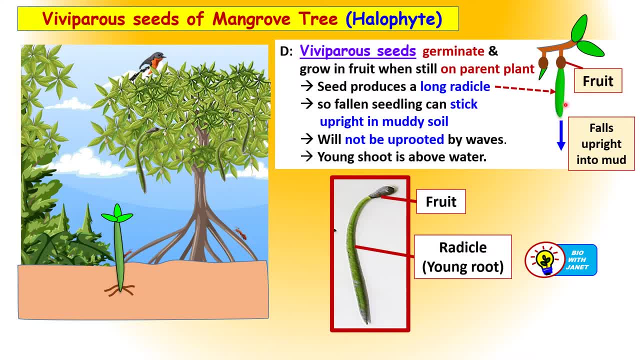 Radical is a young root that grows out from the fruit, So the seed has germinated, It's become a seedling. So seed produces a long radical, so that the fallen seedling, if it falls to the ground, it can stick upright in the muddy soil. 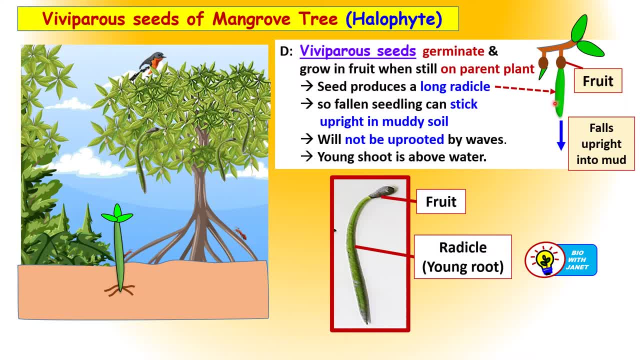 because this radical is quite hard And it will cause the seed to stick upright in the mud So it will not be uprooted by the waves. And the young shoot is also above the water because the radical will hold it upright above the water. 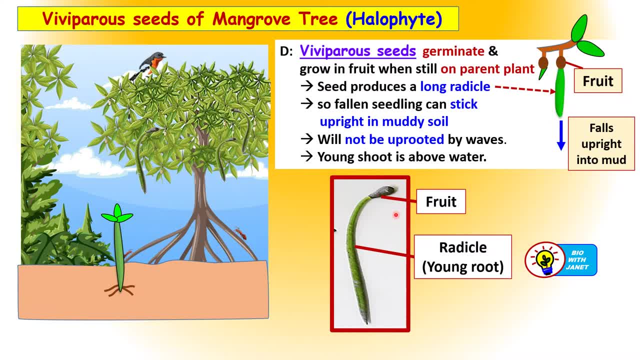 So here we have the real seed which I brought back from the para expedition, And you can see the fruit here, And then you have the radical, Which is the young root. So this radical, it was already on the ground, so I took it up. 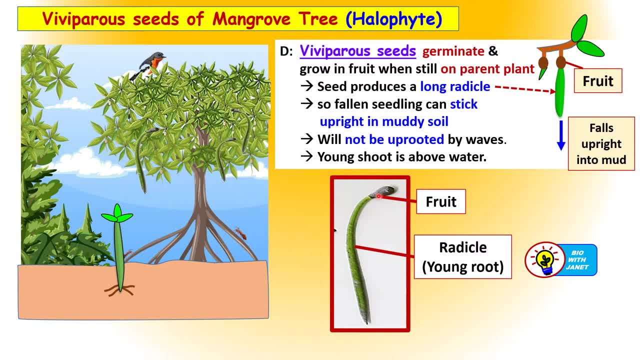 And it is about 0.7 meters long around. that It's very long and it's quite hard. So when it drops to the ground, into the mud from the tree, it can stick upright above the ground and above the water also. 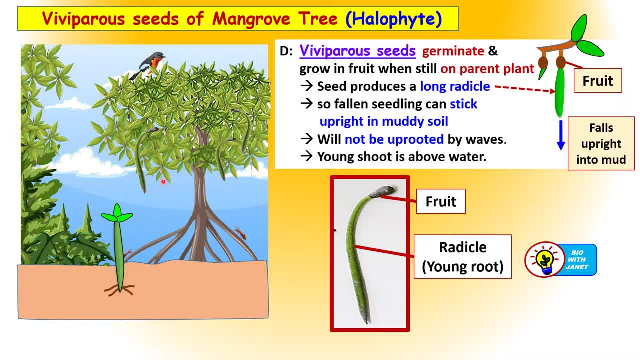 Okay, let's have a look at this Now, because there's high tide and low tide, right? So let's assume it's low tide Now. can you see this fruit here? So, after the seed has germinated and formed a long radical or root here. 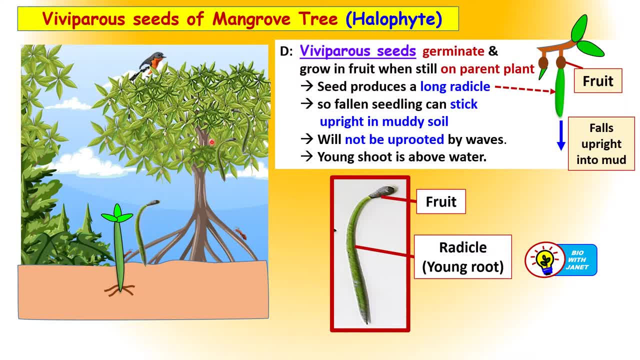 it will drop off from the tree like this- Okay, like this, drop off from the tree. And once it drops off from the tree, it will start to grow roots, like what you see here, And the shoot will grow out. Now, in case there is water. 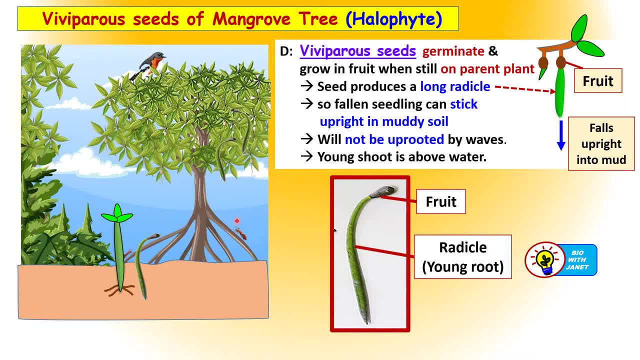 during high tide, the part of the plant will be covered by water. The shoot of the plant, of the seedling, will be above the water, So it will not decompose or rot And the shoot can continue to grow and carry out photosynthesis. 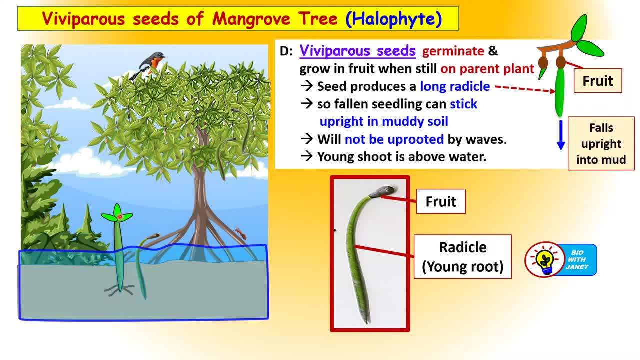 So this will lead to the survival of the mango plant. Also, if the seedling were to fall when there is high tide, then the seedling will not drop directly into the mud, It will float like this. So when it floats like this, it can be carried by the waves to another place. 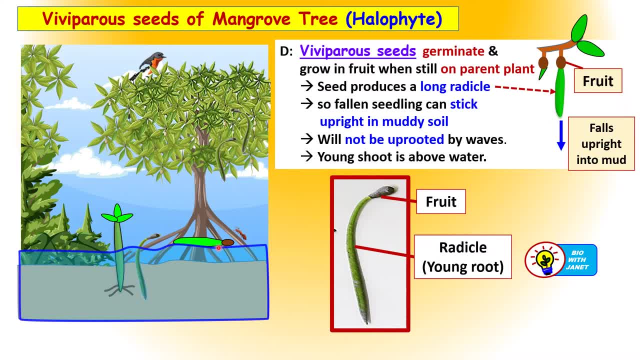 where it will start to grow again So they can colonize another place. All right, So basically we have to know the advantage of the viviparous seeds here, in that they germinate while still on the parent plant and they grow the long radical so that when they fall to the ground 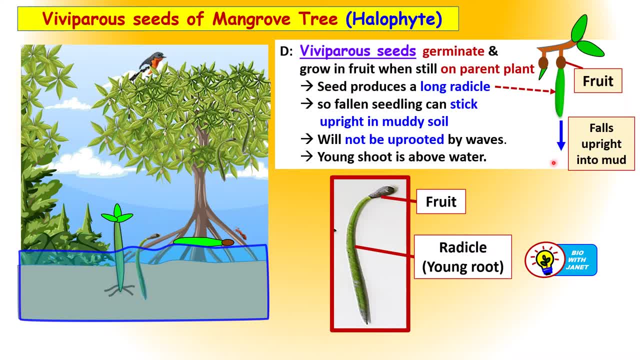 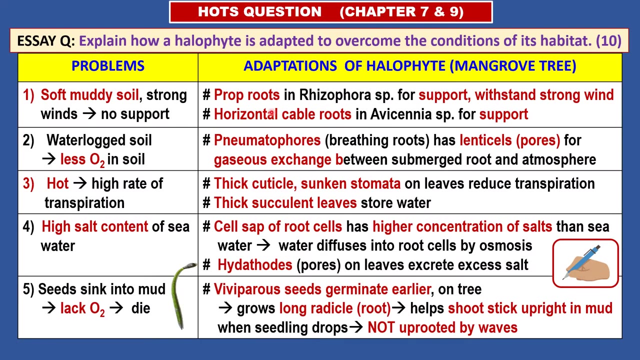 the seedling will stick upright in the muddy soil and will not be uprooted by the waves. Then the shoot is also above the water, so it will not rot. Let's look at a good hots question here which is related to the mango plant. 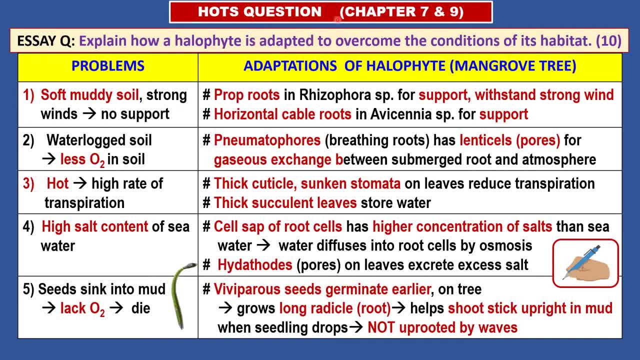 It's related to the mangrove trees, which are halophytes. So this hots question is related to our chapter seven here, which we are discussing, and also chapter nine on the mangrove ecosystem. It can be asked in the SPF. 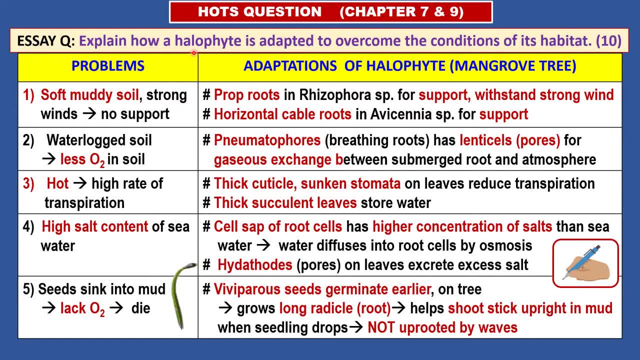 Now the essay question is like this: Explain how a halophyte is adapted to overcome the conditions of its habitat, 10 marks. So explain how a halophyte. So halophytes live in the swampy areas, And examples are the mangrove trees which we have discussed. 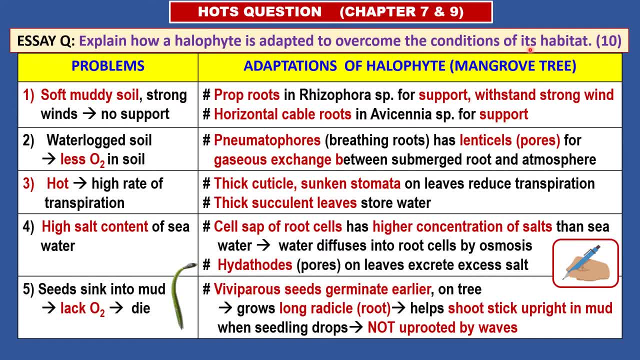 And then how is it adapted to overcome conditions of its habitat? So the conditions of its habitat are challenging conditions such as hot climate, soft, muddy soil and so forth. So you have to mention the conditions of the habitat And after that you have to explain the adaptations or the characteristics. 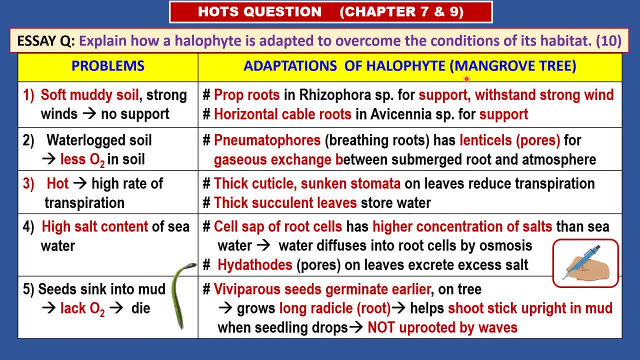 special characteristics of the halophytes, such as the mangrove trees, Right, So here I've got the mangrove trees. I've put the five problems on one side of the table, and then the adaptations to overcome the conditions of the habitat on the right-hand side. 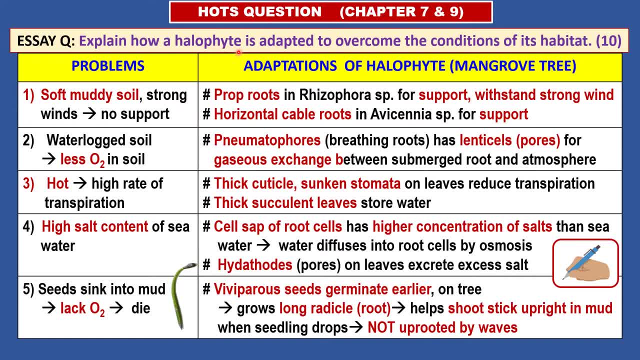 However, in the exam, please do not write a table for this type of question. You have to write it in the form of paragraphs. Okay, So one paragraph each for one problem and its adaptation Table is only used to compare the differences. 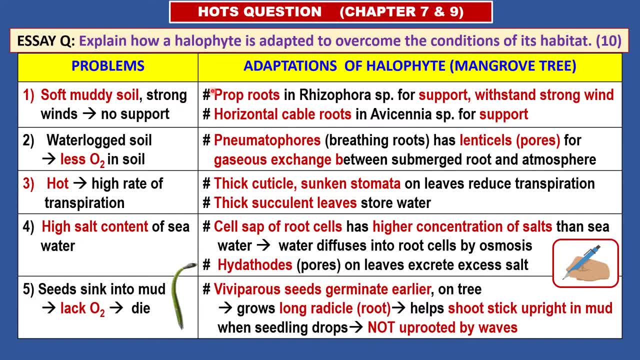 Between two items, two things, All right, So don't use table. But here I'm using table because we are writing it in the form of notes, So it's easy to memorize in this format. All right, In the exam, please write in paragraphs. 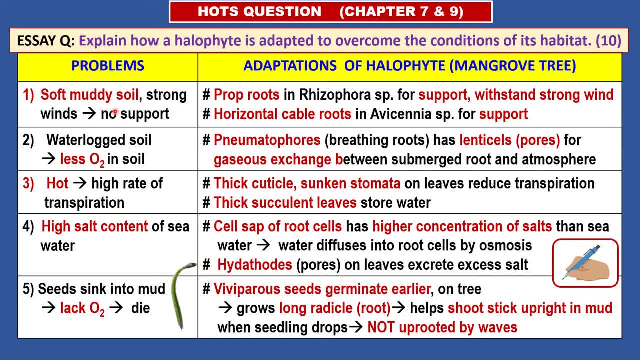 Okay, Let's look at the first problem: Soft, muddy soil in the swampy area and there are strong winds, So the trees do not get any support and they may topple over, They may fall. So adaptations of the halophytes, such as mangrove trees, are that. 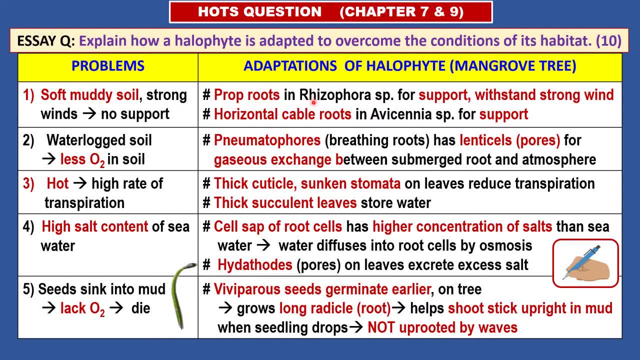 they have prop roots, such as found in the Rhizophora species, which is for support. So these prop roots spread out to form a broad surface area underneath And this helps the plant to withstand the strong winds. However, there's another adaptation, not mentioned in the textbook but still important. 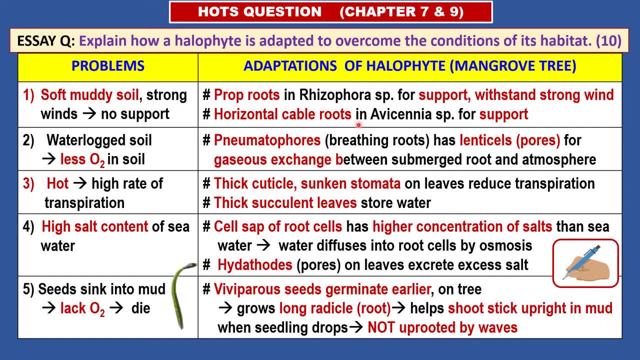 And we need to know the second adaptation in case it comes out in the objective section. So cable roots, Horizontal cable roots in every senior species also give support. However, in the exam please write the prop roots as the most important one. Okay. 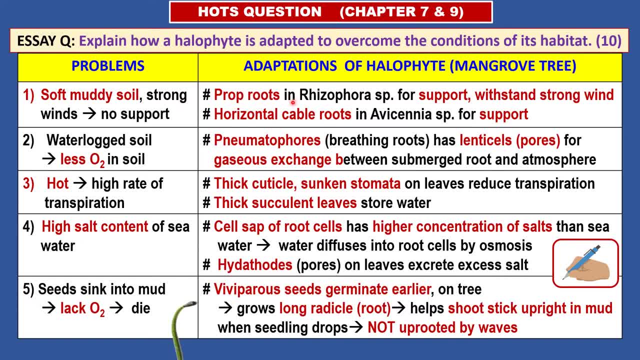 Prop roots for support to withstand the strong winds. Now waterlogged soil. So the swampy area has waterlogged soil or mud with less oxygen in the soil. To overcome this problem, the halophytes have pneumatophores, which are vertical breathing roots with lenticels or pores. 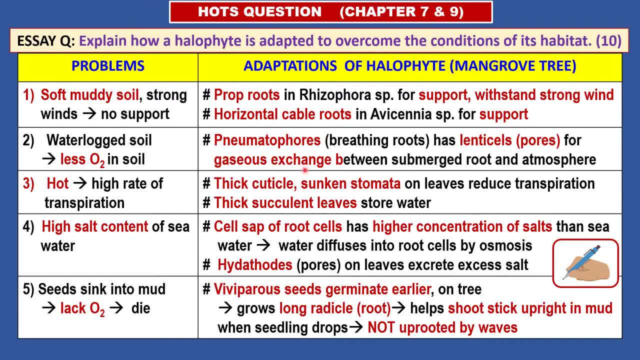 for gaseous exchange between the submerged root- the root that's under the water but which has the pneumatophore sticking out- and the atmosphere. So pneumatophores are above the water and they can carry out gaseous exchange with the atmosphere. 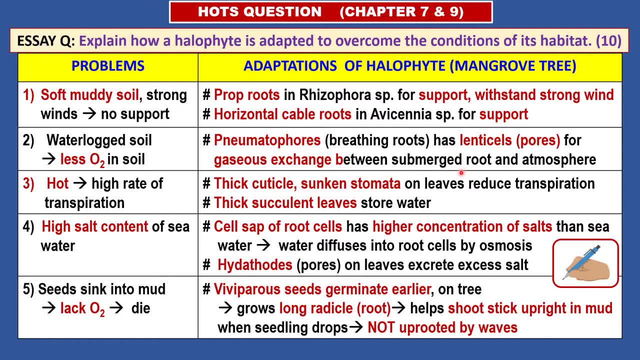 And then the oxygen that has diffused into the pneumatophores can then be, can then diffuse into submerged root underneath. Now number three: hot climate with high temperatures and bright light intensity, So there's a high rate of transpiration or water loss from the plant. 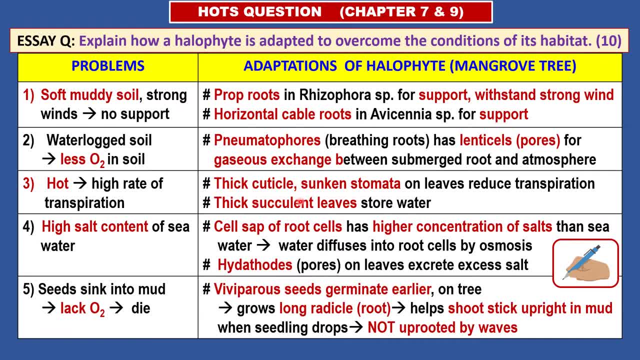 Thus halophytes have thick cuticles and sunken or hidden stomata. hidden stomata or embedded stomata on the leaves to reduce transpiration. Also, the leaves store water, So they are thick and succulent. Next problem: high salt content of seawater may cause the plant to lose water through osmosis. 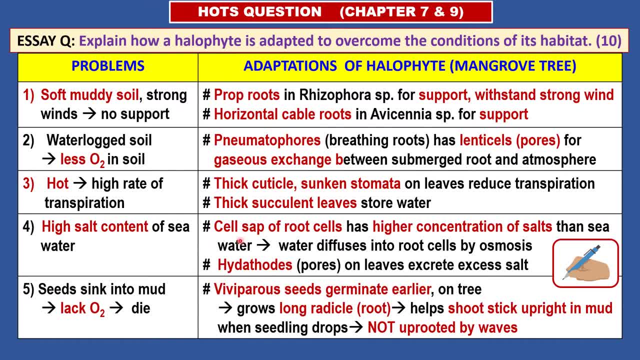 However, for halophytes like mangrove trees, the cell sap of the root cells have higher concentration of salts than the seawater. They are hypertonic to the seawater. The cell sap is hypertonic to seawater. thus water diffuses into the root cells by osmosis instead. 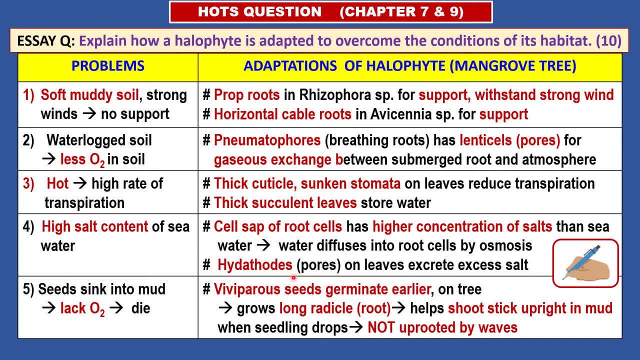 Instead of out of the root cells, water diffuses into the root cells by osmosis. Next, hydratodes, which are pores on the leaves, help to excrete the excess salt from the plant. The last problem is that seeds. if the seeds were to just drop into the mud, 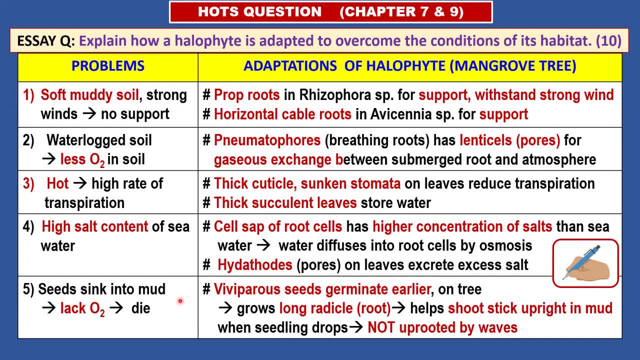 they will sink inside the mud, which lack oxygen, So they cannot germinate. They need oxygen to germinate. So if they can, they don't have enough oxygen. they cannot germinate and they will die. So for halophytes like mangrove trees, they need oxygen to germinate. 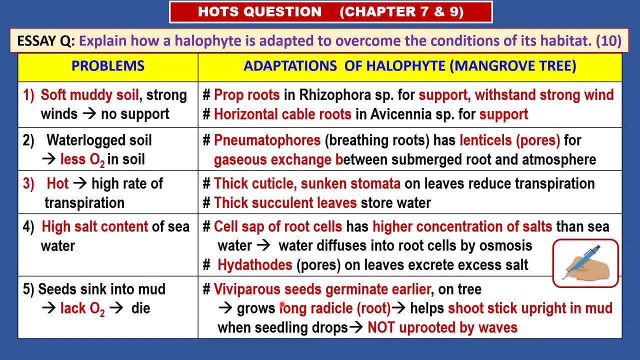 So for halophytes like mangrove trees, they need oxygen to germinate. So for halophytes like mangrove trees, they need oxygen to germinate. They have viviparous seeds that germinate earlier on the tree, the parent tree itself. 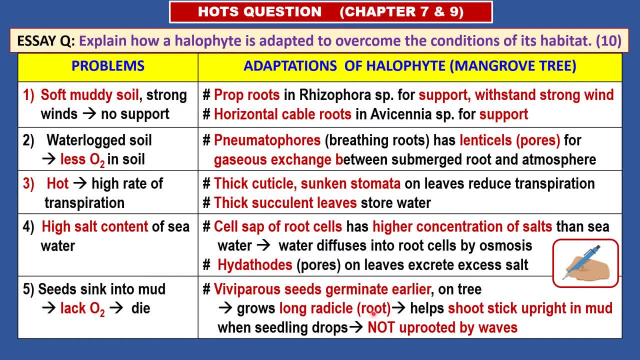 by growing a long radical or root which is very firm. When the seedling drops to the mud, the root will help the shoot to stick upright in the mud so that it is firmly inside the mud and the roots are firmly in the mud and it will not be uprooted. 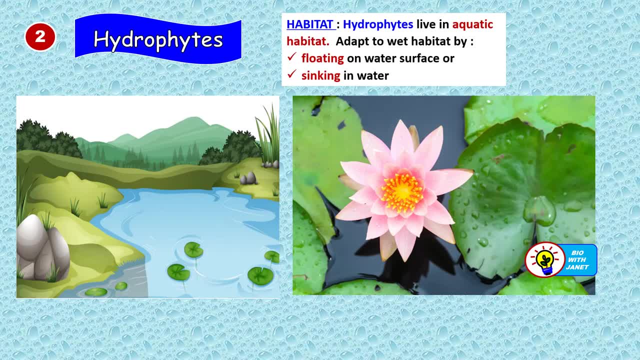 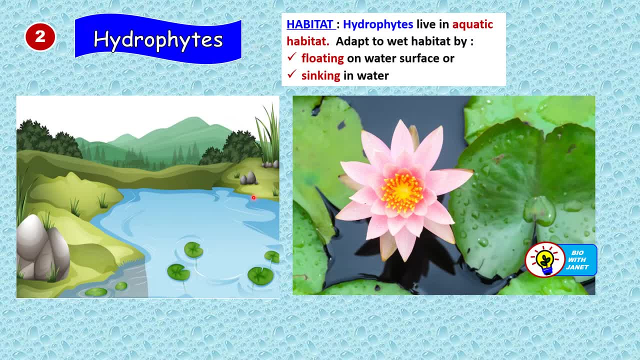 The second type of plant based on its habitat are the hydrophytes. habitat of the hydrophytes are watery environment, wet and habitat, and they grow by floating on the water surface, like the water lilies and the Lotus. so this is a water lily here and they can also. 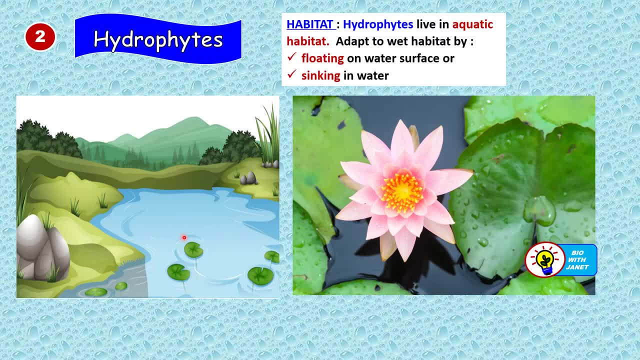 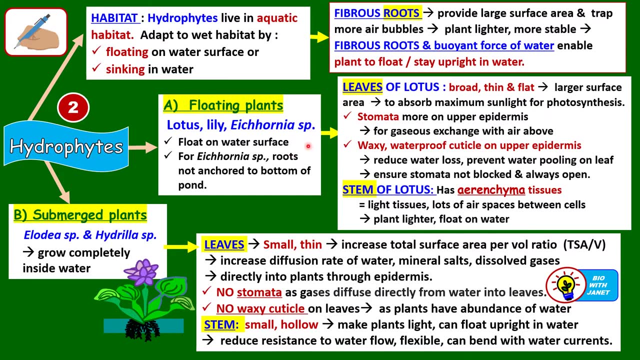 sink. they sink in the water. they can be submerged underwater like hydrilla and elodea species. so here are the notes, or the schematic diagram for the adaptations of hydrophytes to live in the environment. alright, so we're going to look at two types of plants. the floating plants, such 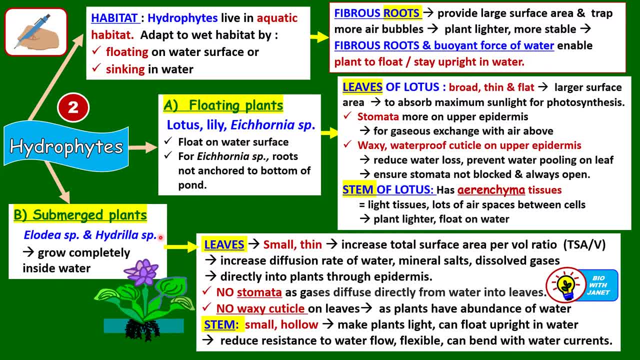 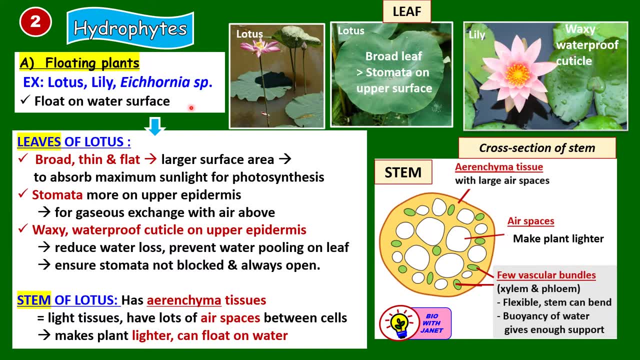 as Lotus, Lily and Echornia species, and submerged plants such as elodea species and hydrilla species. so let's discuss them one by one, start starting with the floating plants. so the floating plants are, for example, Lotus, Lily, lily and aconia species. they float on the water surface. now for aconia species, they have no roots. 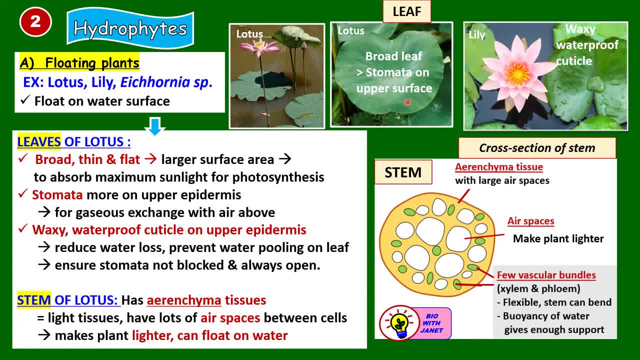 attached to the base of the pond, but for lotus and lily they have. so here we see the lotus and the lily plant. they are different. lotus and lily plant are different because now lily plant, they have leaves with a v-shaped notch here. okay, so the these shaped leaves are notched and split. 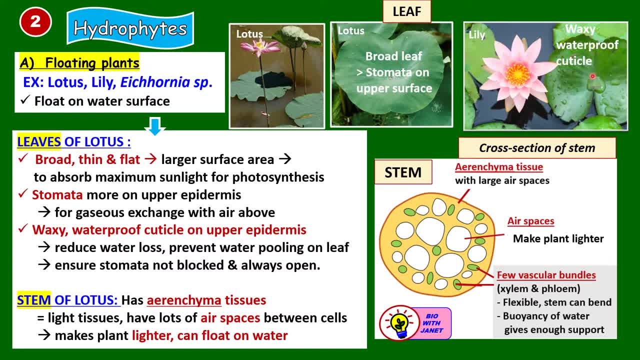 at the stem to the stem here in a v-shape. you see a v-shaped notch here in the center. that's a lily plant and they float. the leaves will float on the water surface. for lotus plant, the leaves tend to be raised above the water surface, and also the flower also, and they don't have the 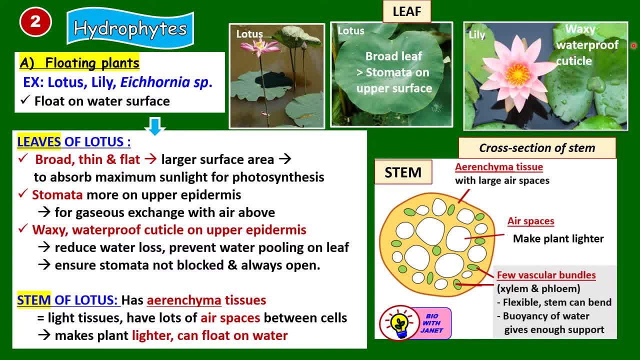 v-shaped notch in the center of the leaf, like this right. so this is a lotus leaf and this is a water lily leaf. both of them are floating plants. now let's discuss the lotus. the lotus has brought thin and flat leaves like this one here, and it provides a larger surface. 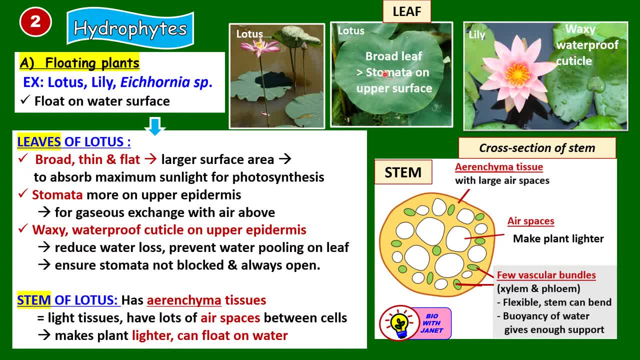 area to absorb maximum sunlight for photosynthesis, so they are very big leaves. then, uh, their stomata more on the upper epidermis than the in the on the lower epidermis. so stomata are paused to allow for gaseous exchange with the air above so that oxygen can diffuse- sorry, carbon. 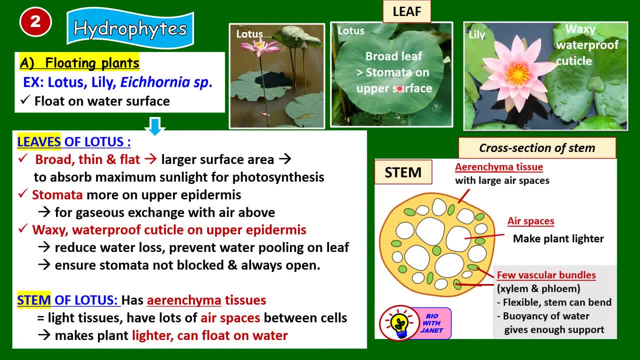 dioxide can diffuse into the plant for photosynthesis and oxygen can diffuse up in the daytime. Now these plants also have waxy waterproof cuticle on the upper epidermis here to reduce water loss, prevent water pooling on the leaf, so that the stomata are not blocked and the stomata are always open. So if water were, 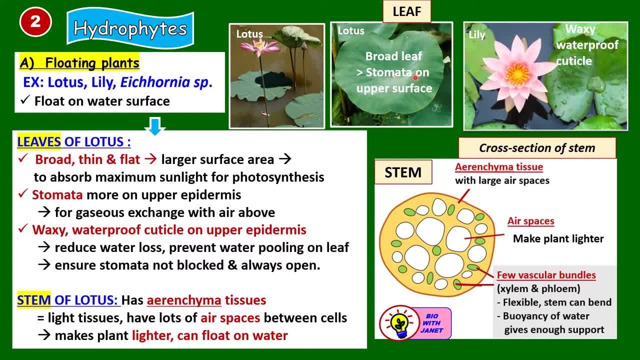 to be splashed on the lotus leaf. they will accumulate in little droplets and they will not form. they won't spread out and then close up the stomata. If the stomata is blocked by the water, then it cannot allow carbon dioxide to enter the leaf for photosynthesis, So it has a waxy. 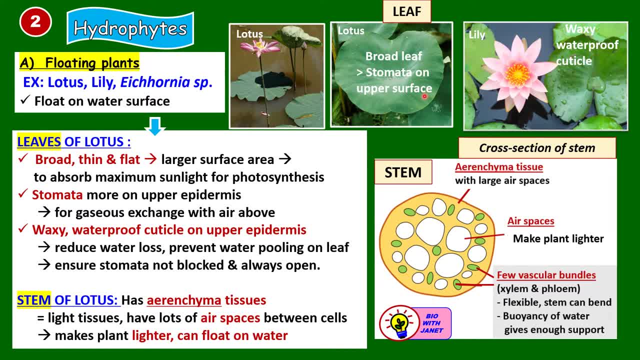 waterproof cuticle to reduce water loss and prevent the water pooling on the leaf. Now let's look at the stem. So the stem is also very important. The stem is also very important to us because the stem has a lot of air spaces inside it, As you can see here, all these white 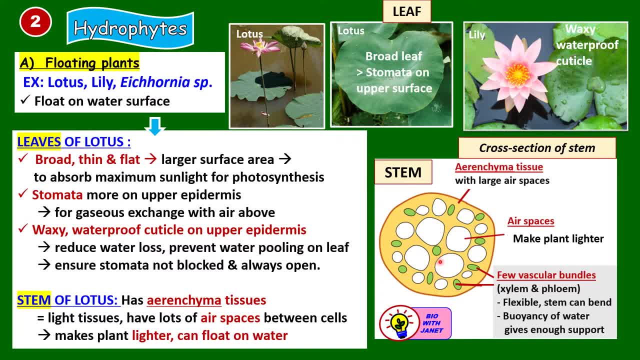 parts are the air spaces and this makes the tissue very light, with lots of air spaces between the cells so that the plant is lighter and it can float on the water. So this type of tissue are called arenchyma tissue from the word air, and there are also vascular bundles in 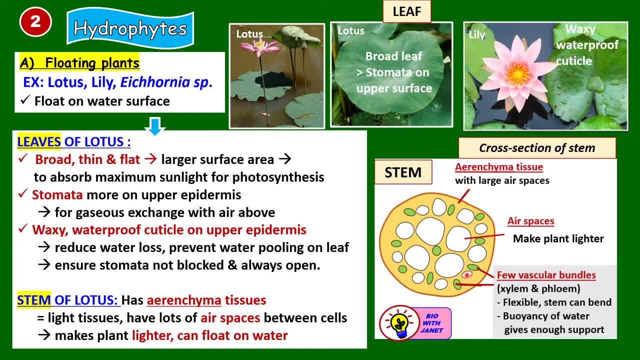 the stem. These are also vascular bundles, but they are not that many, they are few. For example, they don't need a lot of xylem because there is enough water surrounding them. Because of the small number of vascular bundles, the stem can bend more easily. so it's 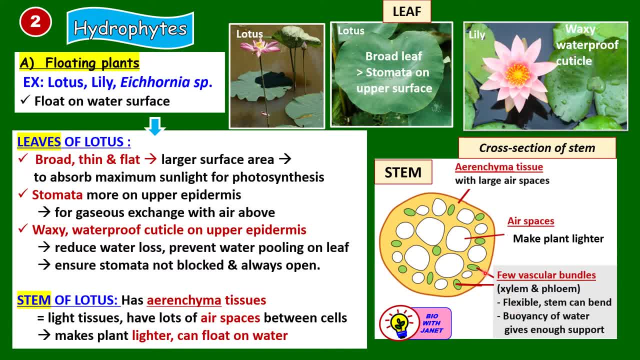 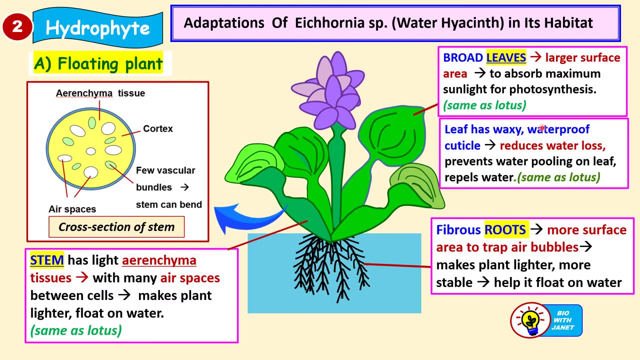 more flexible and especially it needs to bend when there are waves, the river or pond, now when the water is moving. so buoyancy of water gives enough support to to the stem and the leaves to support the stem and the leaves. this is another type of floating plant which is aconia species or water hyacinth. 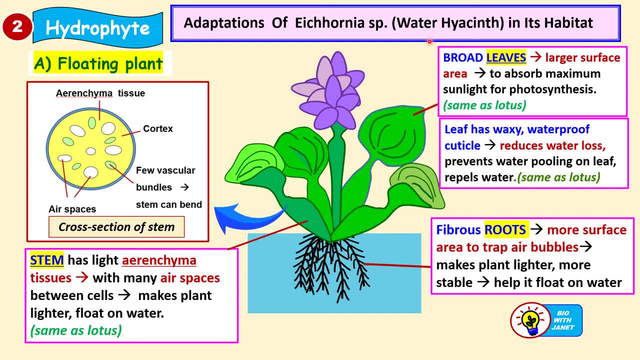 which we have discussed in the topic of phytoremediation, right? so here we are going to discuss is adaptations for living in its habitat now. so a corner species. now, this is not mentioned in your textbook, but i would like to give you a few, a few points here, in case you can. is asked as a hot question. so if you look at this plant, what? 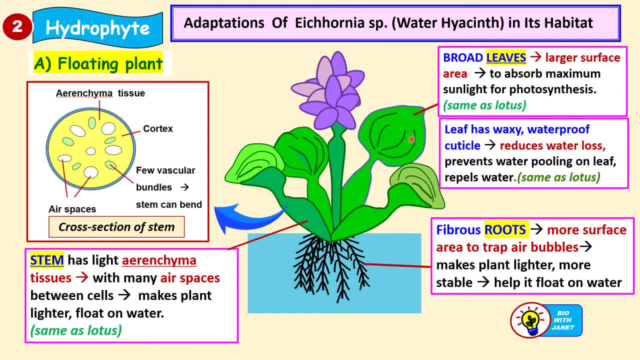 is the adaptation of this plant for its habitat now. firstly, it has broad leaves, so broad leaves provide a larger surface area to absorb maximum sunlight for photosynthesis. and then the leaf is very shiny because it has a waxy waterproof cuticle to reduce water loss, prevents water pooling on the. 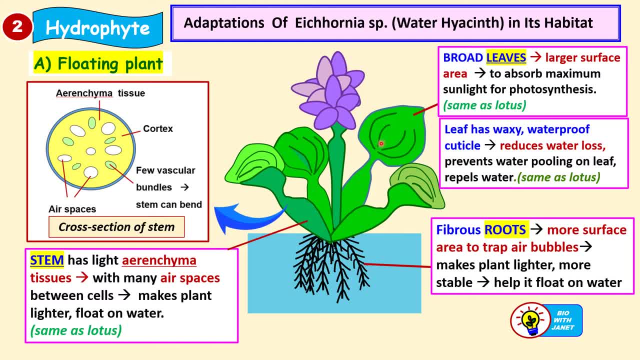 leaf. it repels water so that water will not stick on the leaves and cause the leaves to rot. and then the roots, the stem first. the stem has like erenchyma tissues, as we can see here, something like the lotus plant. it has a lot of air spaces between the cells, so this makes the plant lighter. 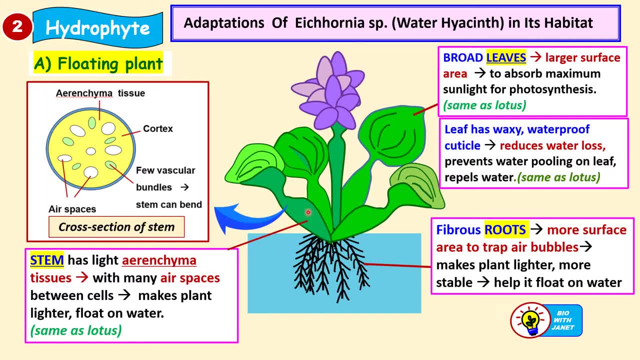 because of the air and then the stem can stand, can float on the water so it won't sink. so it also has erenchyma tissues in the stem, like the lotus plant. then it has very fibrous roots which will increase the surface area of 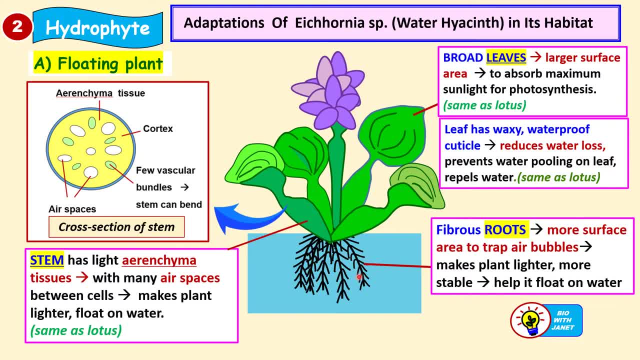 the roots and trap air bubbles in between the roots. so this makes the plant lighter so that it's able to float more stable and lighter to help it float on the water. okay, so these are the adaptations of the leaves. the steps are of the leaves, in any sense of the same basis that you've. seen before. if there are salt buds, then they are great aberrant plants. often they easily worked them. the bran cannot be used and they can flow better. if they受 a lot of water is the stand. it can dampen the leaves. it 얘or that we are actually talking amgood with, or that many of the three Cayman 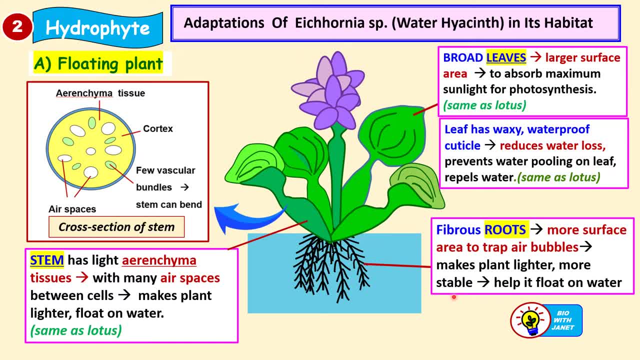 that, i believe, is an extreme condition. okay, so these are the adaptations of the leaves, the stem which has arenchyma tissues, and the roots, which are fibrous and quite dense to trap the air bubbles. So it's very interesting when we look at this plant and we realize that it's very well. 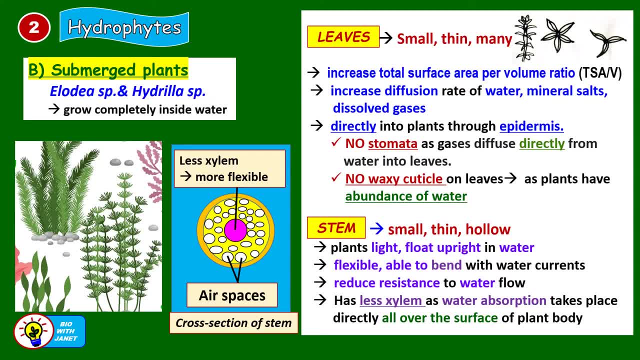 adapted to float on the water surface. Now, just now we discussed the first type of hydrophytes, which are the floating plants, So next in this slide we'll discuss the submerged plants, such as Elodea species and Hydrella species that grow completely inside the water submerged in the 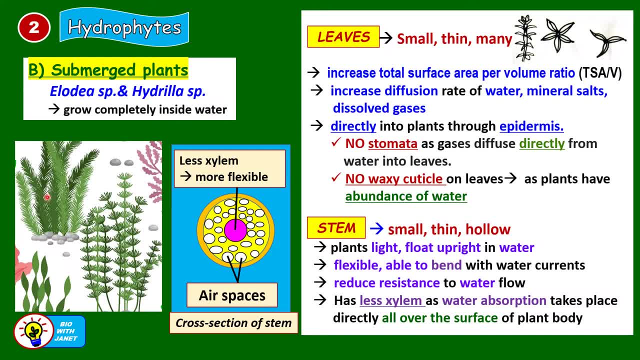 water. So let's talk about the leaves. Now. you can see here, for the submerged plants like this, the leaves are very small, thin, but many, So this helps to increase the total surface area per volume ratio. compared to a few big leaves, It's better to have many small, thin leaves. 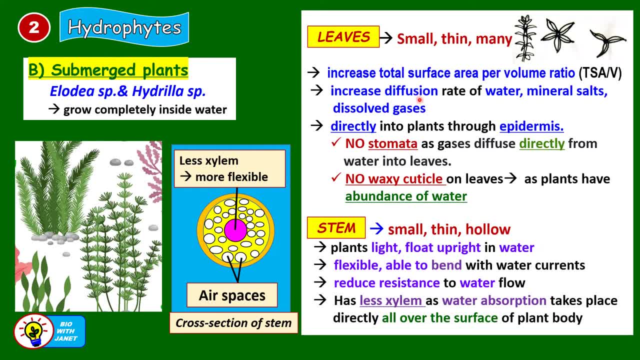 and this will increase the total surface area per volume ratio so that more water can diffuse from the environment, from the water into the plants through the epidemics of the leaves. So large total surface area increases the diffusion rate of water and mineral salts from the surrounding water and dissolved gases from the surrounding. 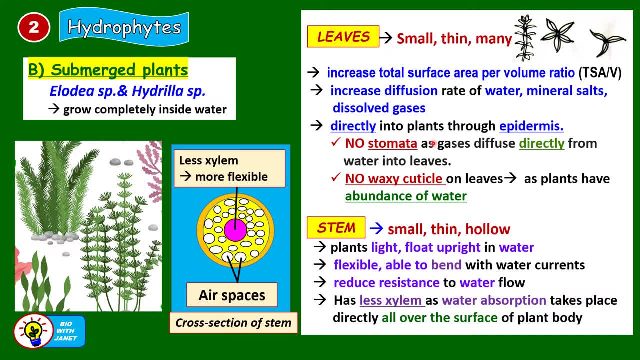 water surrounding water directly into the plant. Now, another fact is that the leaves do not have any stomata, because the gases that are dissolved in the water diffuse directly from the water into the leaves. They don't diffuse from the atmosphere into the stomata, because all these plants are submerged underwater, So the gases are dissolved. 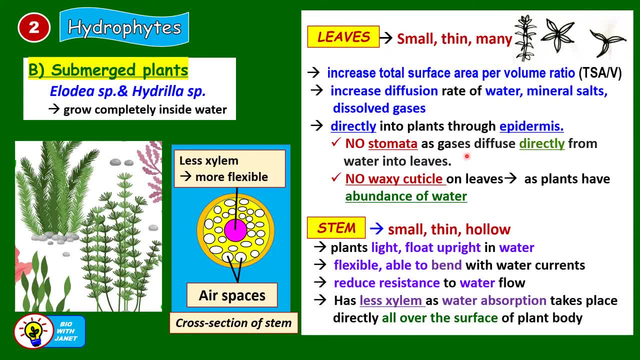 in water and they diffuse directly from water into the leaves. So this is a very important thing to keep in mind when you're looking at hydrophilic hydrophilic plants. So let's talk about the leaves. So this is a very important thing to keep in mind when you're looking at hydrophilic plants. 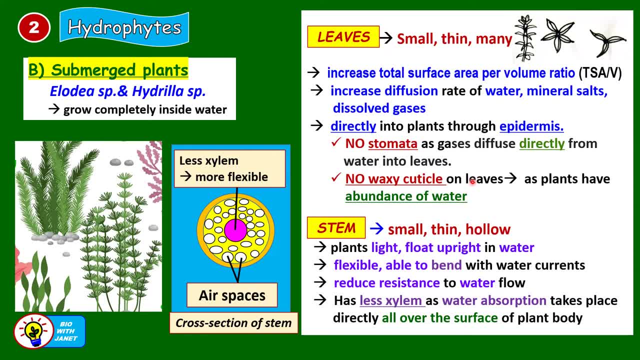 It addresses the resistance of nitrogen from the bud to the stem cells, such as taking an effective exposure period f ziemlich all the leaves- and Kathy said that 최ñoséply- such as the squelney concept and also other factors请 said, because this is not about fire, colipres or baking of inorganicques. 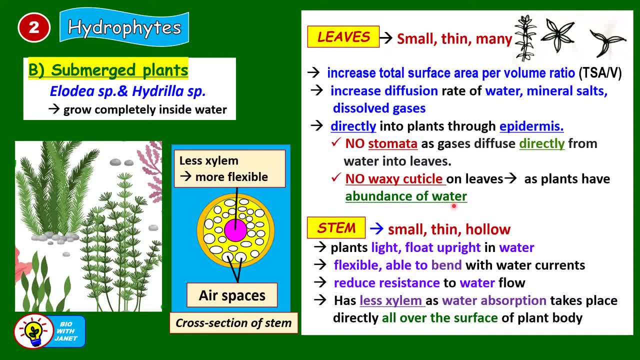 We also have to keep in mind when we treat plants. it has to beful treated with信もう from water into the leaves through the surface overall or the surface of the leaves. Secondly, there's no waxy cuticle on the leaves. now, how about the stem? so again, the stem is small and thin and it is hollow. now you can see here it. 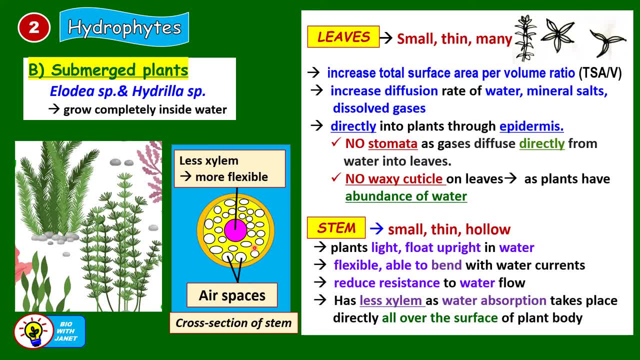 has a lot of air spaces too, just like for the floating plants, all right, just like for the Lotus. so it has a lot of air spaces and the stem is quite hollow full of air spaces. then this makes the plants very light so that they can float inside the water, upright in the water and with 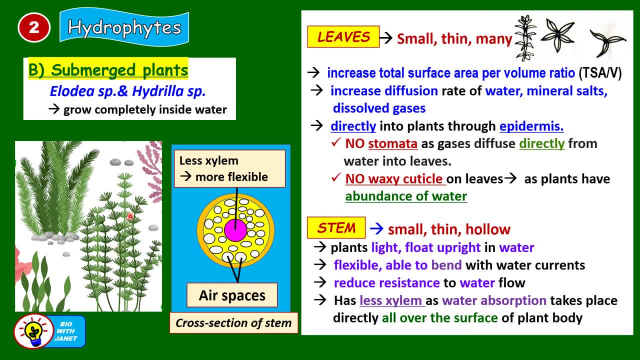 the buoyancy of water also to help them float upright. however, if you pull them out from the water, take them out from the water- they will collapse. right, because they don't have the buoyancy of water to support them anymore. right, so the stem is also flexible because it has less. 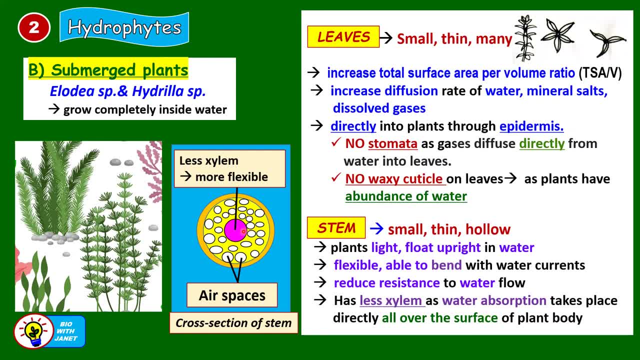 xylem. the xylem is found the center part of the stem only and this xylem is what makes the stem rigid. so when there's less xylem, the stem is more flexible, not so rigid, and it's able to bend with the water currents. now, when the water currents are moving, 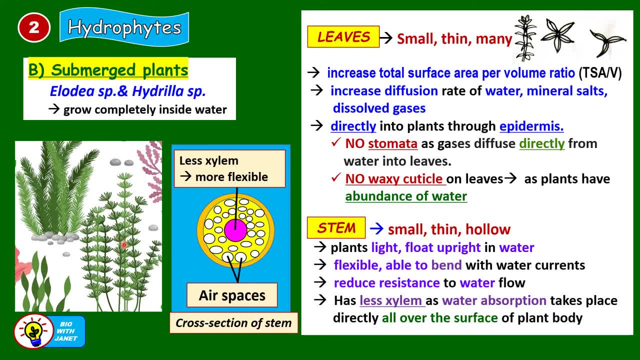 the stem will not break, but it will just bend along with the water currents right and in this way it will reduce resistance to the water flow so that the stem will not break like a stiff stem. like for land plants. the stem is very stiff and if the 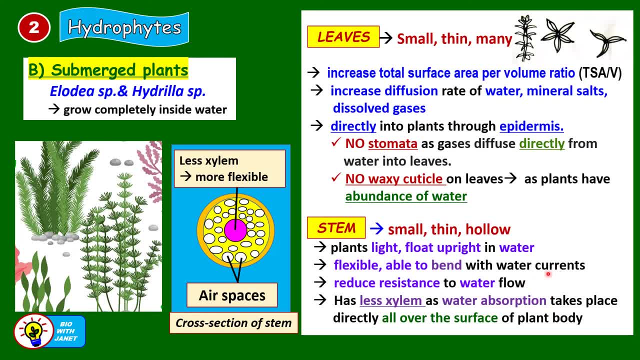 you put the stem into the water. if the water current is very strong it can break the stem. but for the submerged plants, they are very flexible, they have less xylem, they are more flexible and they'll just bend with the water currents. all right, so less xylem. there's less xylem in the 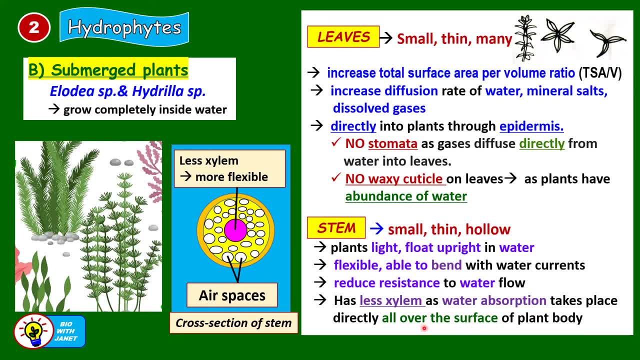 stem. also because water absorption takes place directly all over the surface of the plant body. the plant does not need xylem to transport water from one place to the next. it absorbs water directly from the whole surface of the plant body through the leaves to the stem. 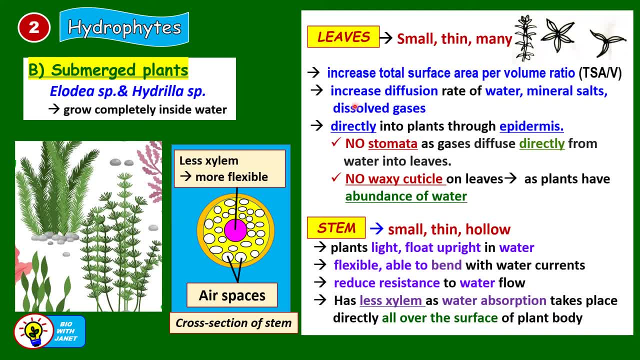 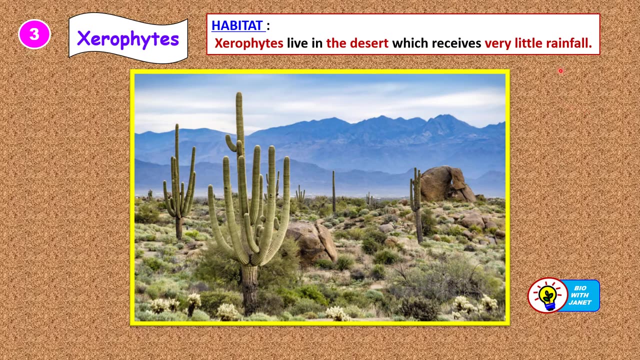 through the leaves and the stem. all right. so these are the adaptations of the submerged plants that look like very have, that have very small thin leaves and, uh, also very small thin hollow steps. now let's look at xerophytes, which live in the desert. that's very hot and receive very little rainfall. 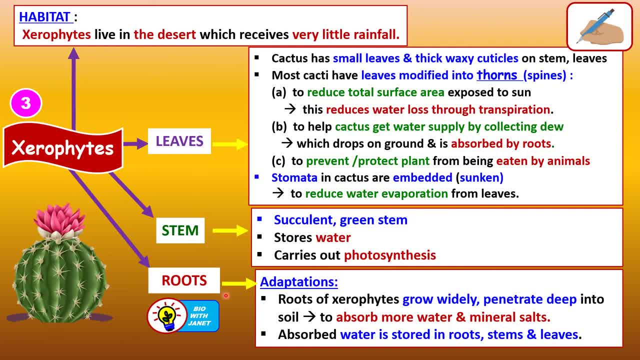 so we're going to discuss the, the adaptations of the leaf stem and the roots again. so all this will be discussed in the next slide. let's have a look at the, the adaptations of the different parts of xerophytes. now the first. so here we're going to look at 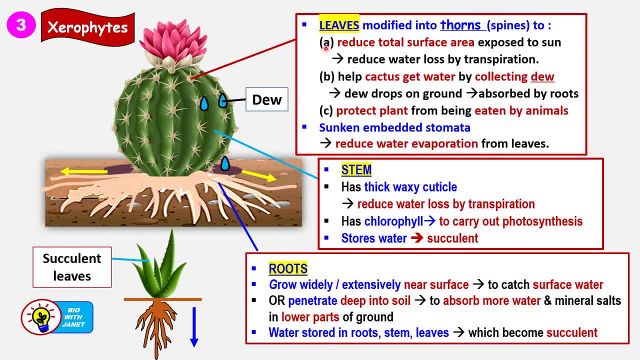 a cactus that is rounded in shape. so what are the adaptations of this xerophyte? firstly, the leaves are modified into thorns, sharp thorns. so this is actually leaves that are modified. normally we call them spines. textbook use the word thorns, so thorns or spines, and that means the surface area of the. 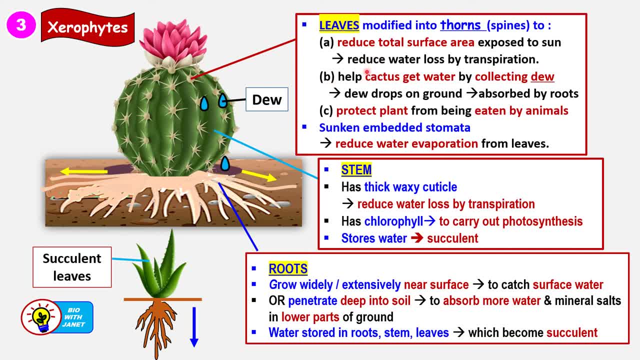 leaves have been reduced so as to reduce the total surface area exposed to the sun. because living in desert is very dry, the plant must conserve water and reduce water loss by transpiration. so because the total surface area of the leaf becomes so tiny, thus water loss by transpiration is greatly reduced. 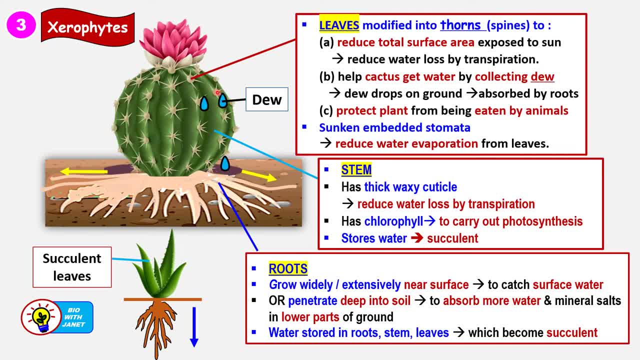 and the thorns also help the plant to get water by collecting dew at night. at night the the vapor, water vapor- will condense on the thorns and then it will drop to the ground and then it will be absorbed by the roots. so these thorns help to collect dew, because the dew will 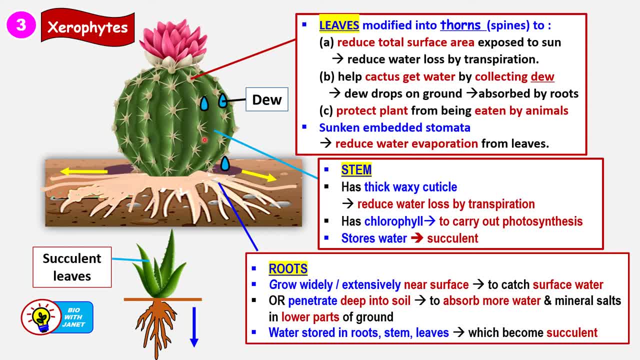 condense on the thorns and they will drop into the ground and be absorbed by the roots. next, these spines or thorns are very sharp, so they will protect the plant from being eaten by predators or animals- animals. Now, lastly, on the leaves, there are sunken or embedded stomata to reduce water evaporation. 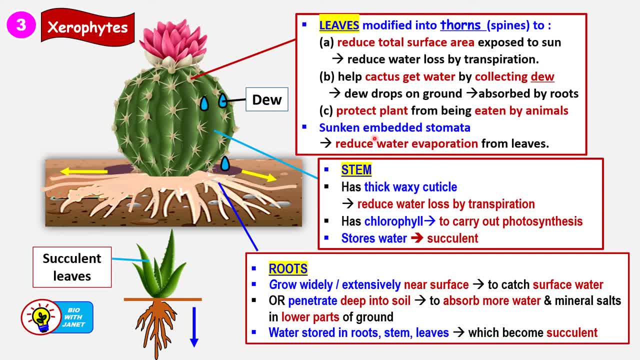 from leaves. So sunken or embedded stomata. Now the textbook use the word embedded and normally the term for it is sunken stomata. So sunken stomata or embedded stomata are stomata that are hidden away inside the leaf, which we'll see afterwards in the next slide to reduce water. 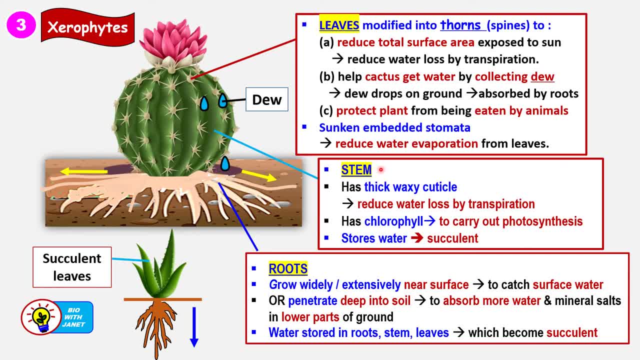 evaporation from the leaves, Now stem. The stem has a thick waxy cuticle and it is very is enlarged here because it stores water. So the thick waxy cuticle makes the stem a bit shiny and that's to reduce the water loss by transpiration. Okay, the thick waxy cuticle, Then the stem is green in color. 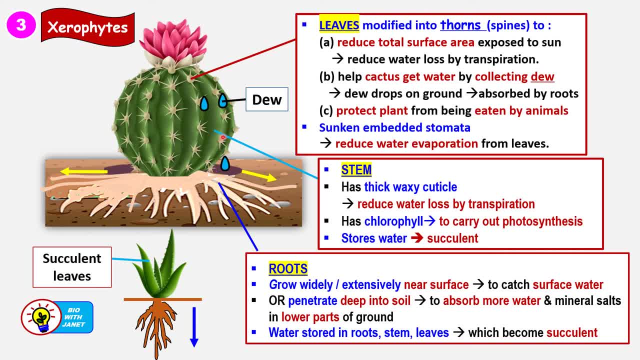 to carry out photosynthesis and produce organic food substances for the plant. So the leaves do not carry out photosynthesis because they're not going to produce organic food substances, They have been reduced to form spines or thorns. It's the stem that is enlarged and able to carry. 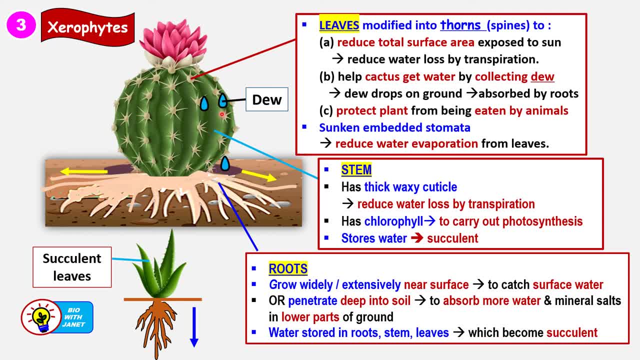 out photosynthesis. So it's green in color and apart from that, most of the stems are swollen or bulbous and that is to store water. So we say that the stem is circular or juicy, full of water. Next are the roots. So there are two types of roots. The first type of 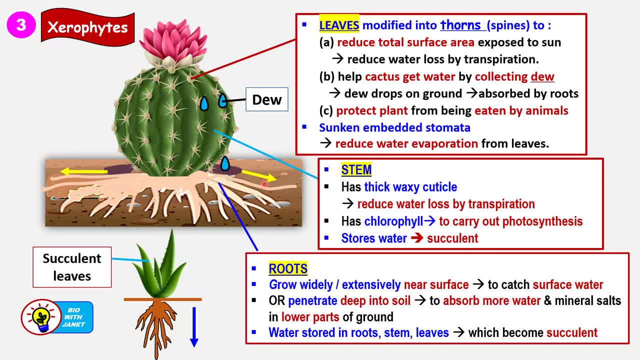 roots grow widely and extend to the leaves. So the first type of roots grow widely and extend to the leaves. So the second type of roots grow extensively near the surface and spreads out. It's widespread To catch the surface water, especially after the rain or during the rainy. 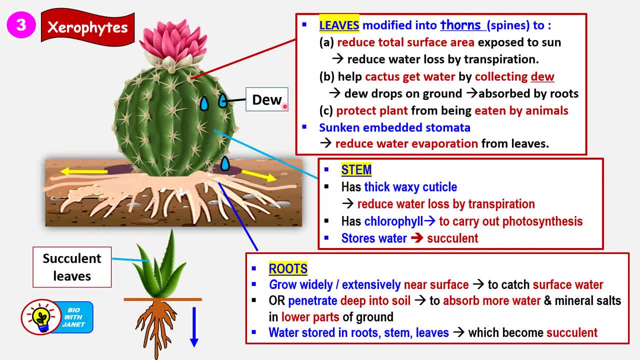 season, which happens very rarely in the desert. So these roots will be available to absorb as much as water as possible from the surface of the ground. But there's another type of root maybe could be in the same plant or for different plants. These roots penetrate deep into the soil, So they 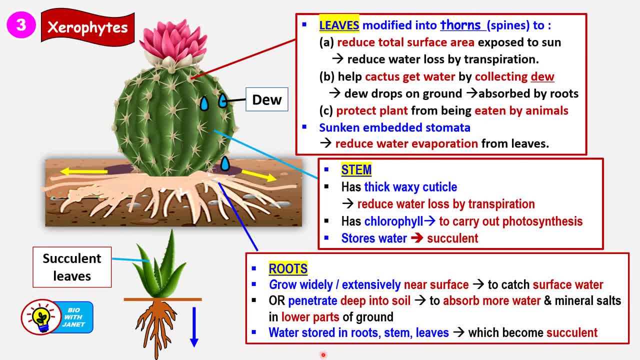 they penetrate vertically downwards into the soil to absorb more water, mineral salts, in the lower parts of the ground. that's not for catching the or for absorbing the surface water anymore, right, it's for absorbing water from the, from the lower parts of the ground. after that, the water is. 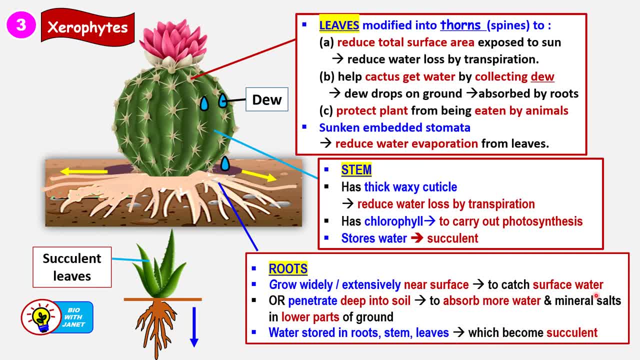 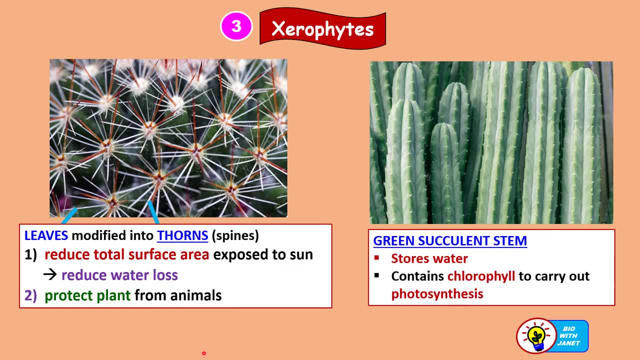 stored in the root stem and leaves, which then become succulent. so let's find out what is a sunken or embedded stomata. so here's a close-up of another cactus, with leaves modified into thorns to reduce water loss and also to protect the plant from animals or predators. here's a close-up of the. 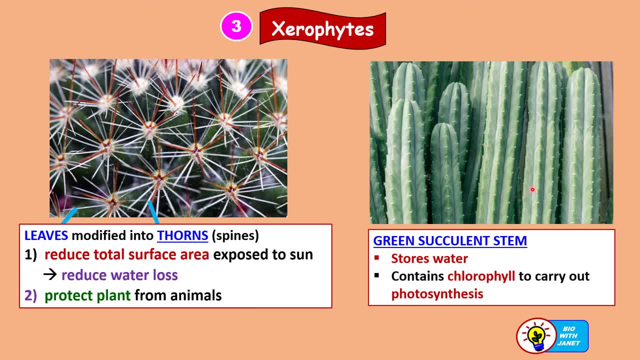 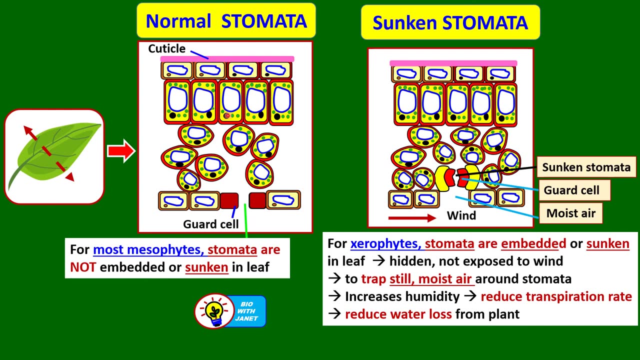 of a cactus stem, which is green and succulent, to store water and at the same time, it has chlorophyll to carry out photosynthesis. now, what is meant by sunken stomata or embedded stomata? so first of all, let's look at the cross-section of a leaf. for most mesophytes, 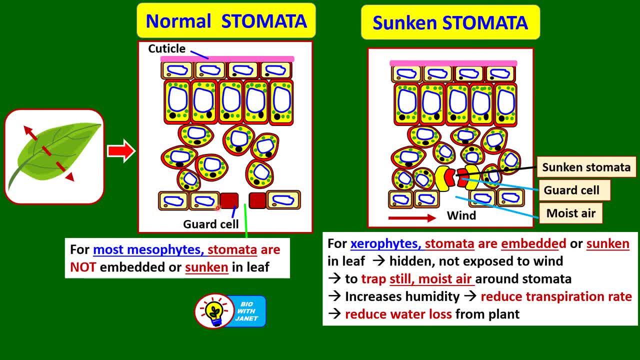 the cross-section of the leaf shows that the stomata is at the same level as the lower epidermal cells. here the gut cells are also at the same level, so the stomata is not hidden away. it's at the same level as the low epidermis and this is the normal position of the stomata. 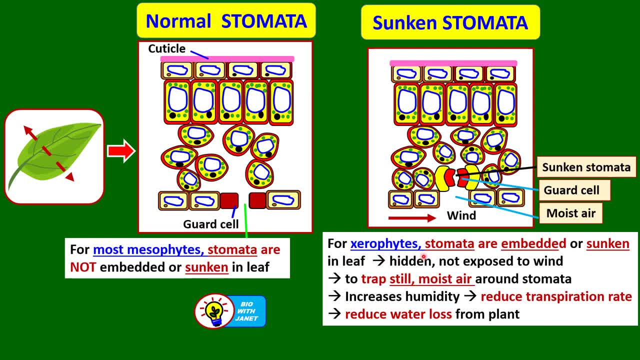 but for xerophytes that live in the dry, hot conditions, they have to reduce water loss through the stomata, so their stomata are embedded or sunken or hidden in a way in the leaf not exposed to the wind that is flowing underneath here. 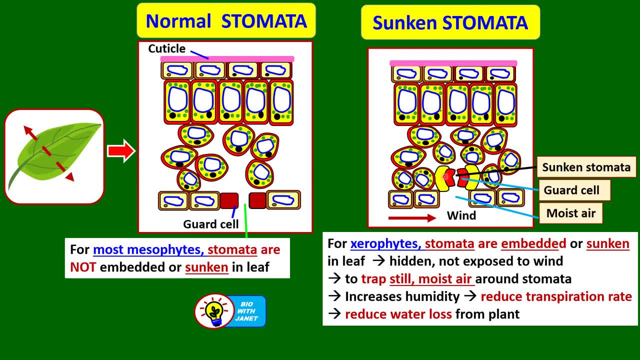 so there's an area here, just below the stomata, that is used to trap the moist air. okay, because the stomata are hidden, are raised inwards, they are found further inwards to the lower epidermis, so this area here will trap moist air because of the 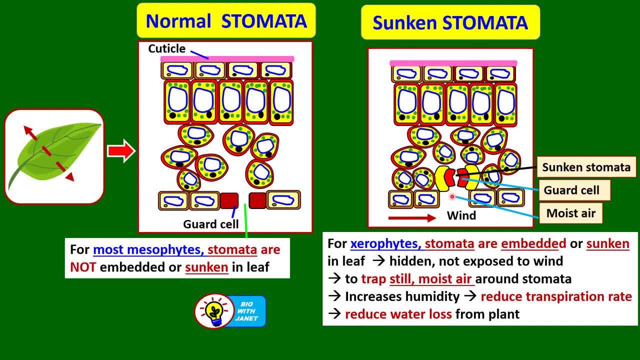 water vapor that diffuses out from the leaf, you. the water vapor will accumulate here and it will not be exposed to the wind. so this will create a condition of high humidity so that less water diffuses out from the inside of the leaf to this area. so it reduces the transfer. 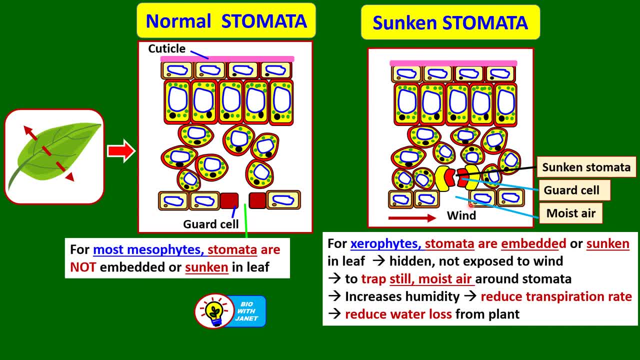 rate and reduces water loss from the plant. right, that's all for this lesson. please share, like and subscribe, and thanks for viewing. till then, goodbye.